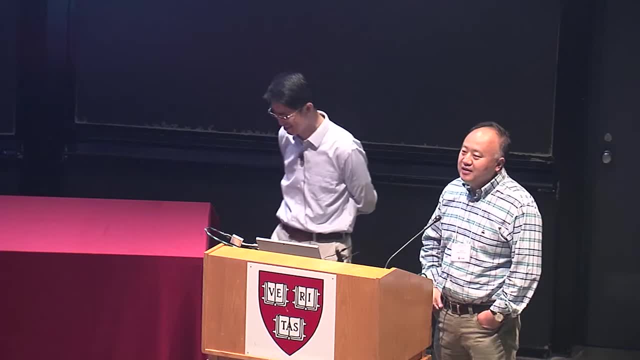 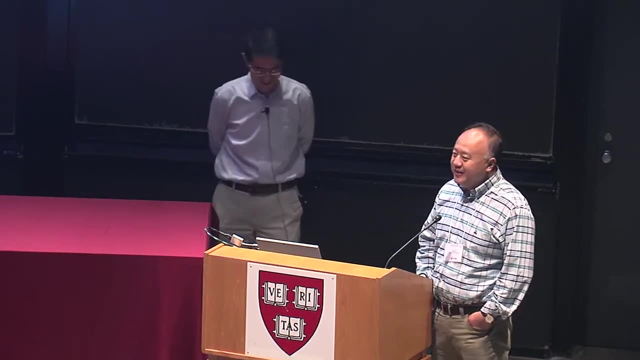 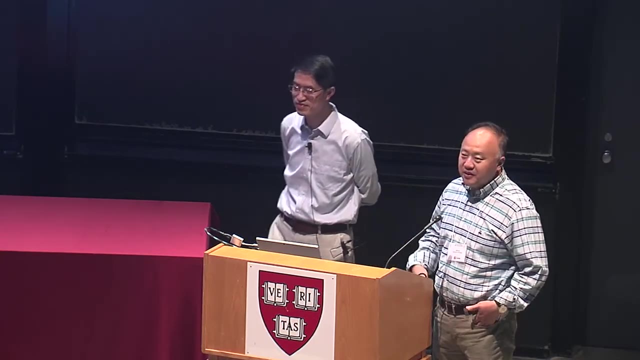 from assistant professor to full professor. The previous one was a famous Arthur Dempster who retired 10 years ago about. So the gap is about 50-some years between the first and second. OK, without further ado, here I give you Professor Samuel. 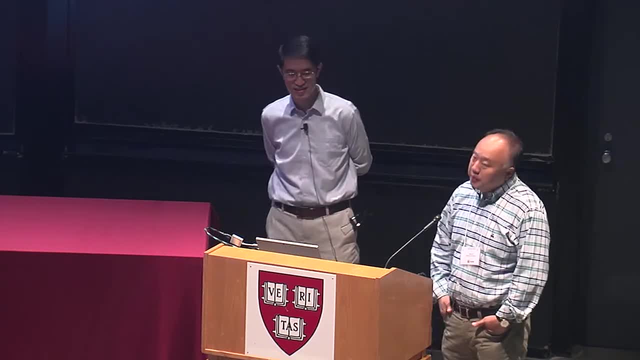 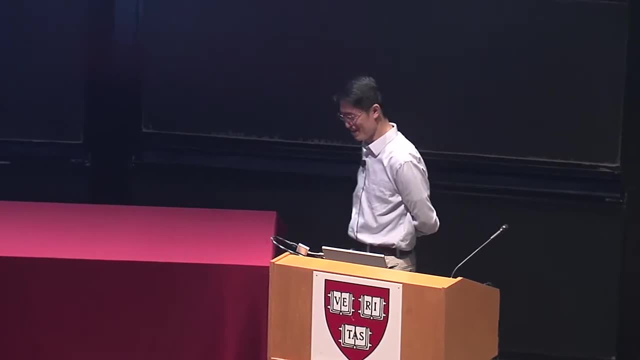 Koh. He will tell us about his work in electronic medical record. Thank you, Can you hear me? Thank you very much, Jun, for the introduction. The second part just says that our department is very small For a long, long, long, long time. 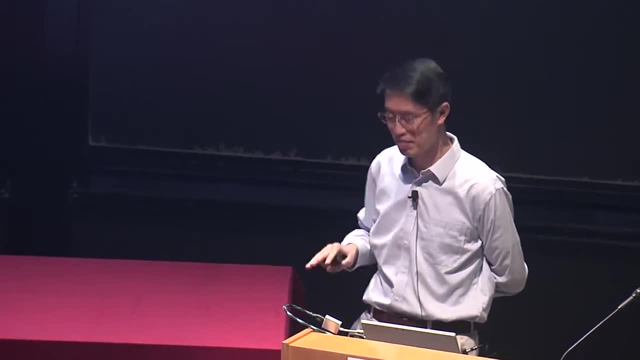 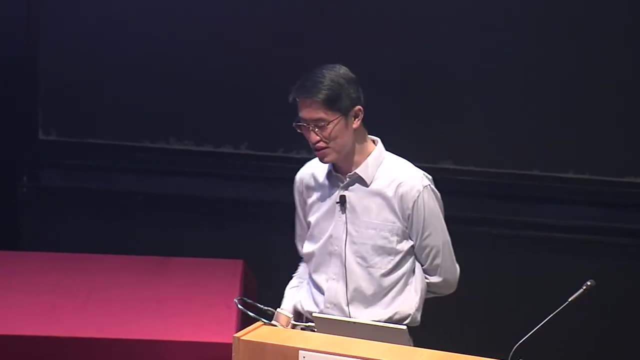 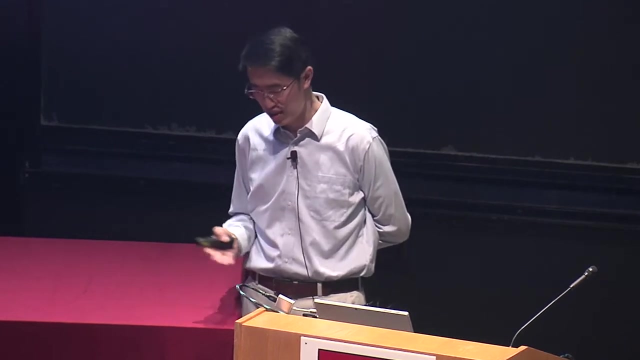 there are only four, three tenured faculty members in the Department of Statistics. That's to put in the context, And so OK, as Jun mentioned, what I'm trying to do today is to give a sort of introduction about our work and our adventure in dealing with electronic health data. 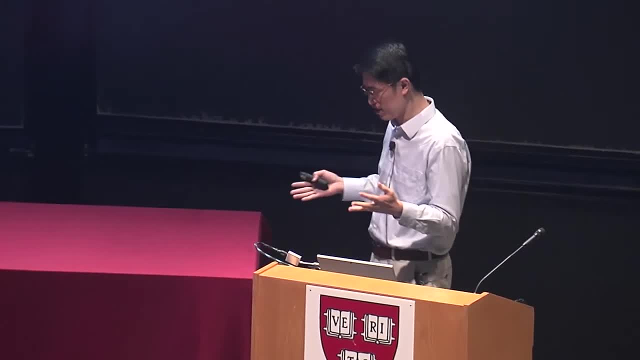 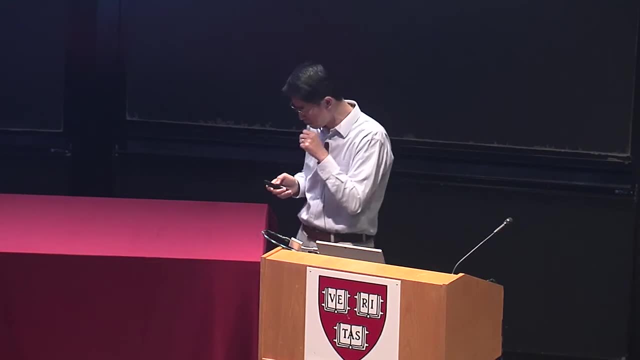 So I'll tell you what we did And what we're looking after, And also some lessons we learned and some insight we gained from this process. So this talk is based on joint work with Shihao Yang, who is currently a PhD student in the Department of Statistics. 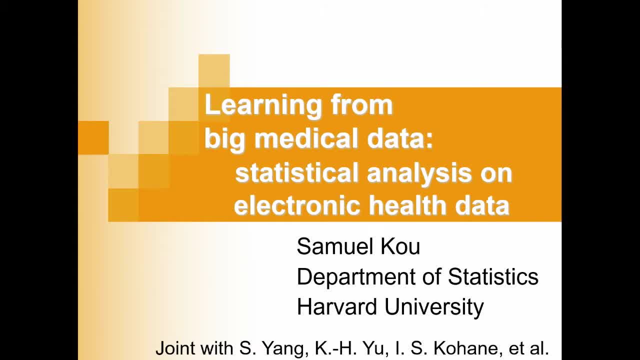 and Kunxin Yu, who is a Harvard data science fellow, and my collaborator, Zach Cahoney in the Harvard Medical School, And you can see there's also other courses involved as well, And so what I'm trying to do is to talk. 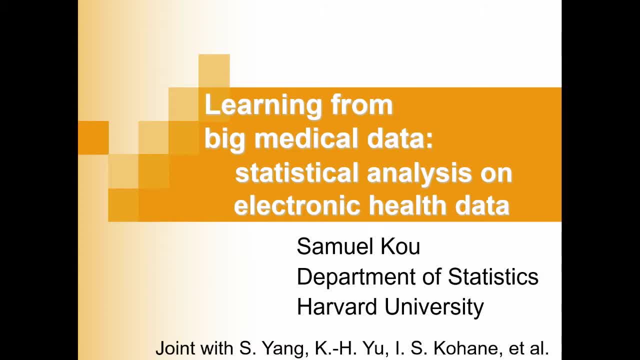 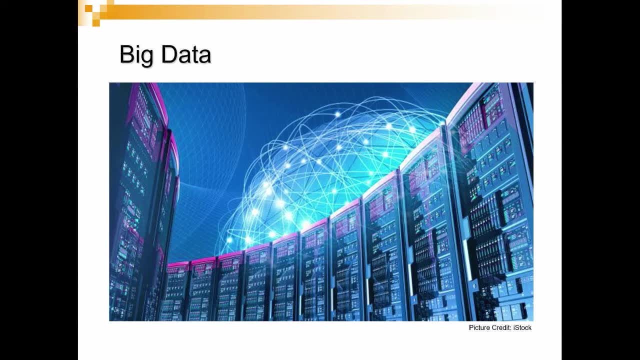 about big medical data, applications on big medical data. So this is a big data conference. Let me say a few words of big data. We all heard of big data And that's why we're here today And, as a matter of fact, whether we like it or not, 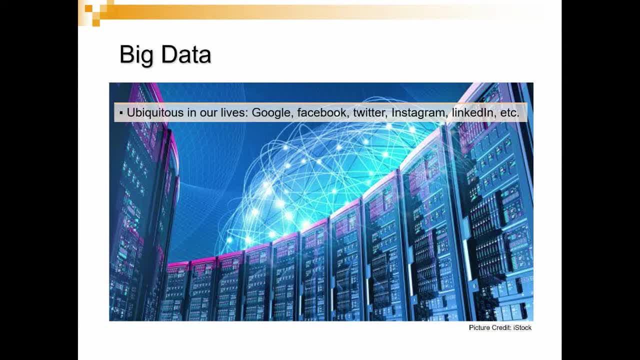 everyone of us pretty much are involved in some big data online platforms one way or the other. For example, when you do Google, when you do Facebook, or when you do Instagram, Twitter or LinkedIn and so on, you already not only participate in the big data. 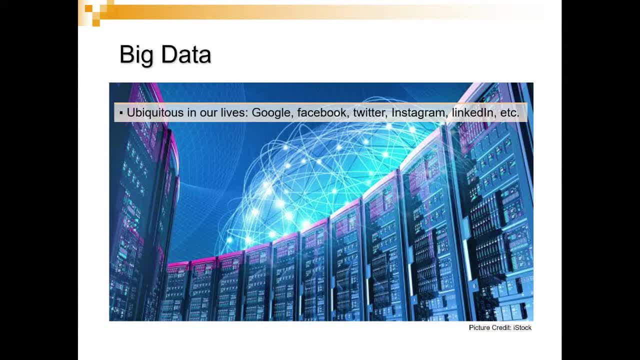 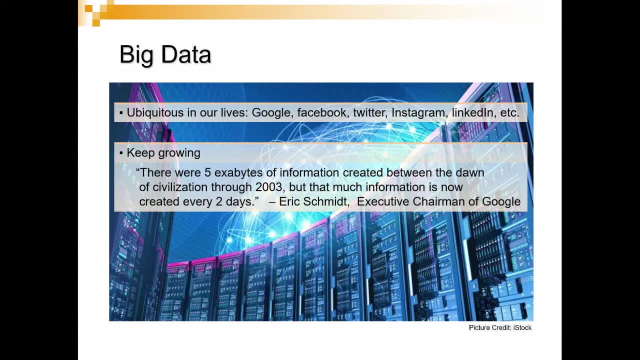 platform, But also we all actually actively contribute our own effort to their data collection. So, as a matter of fact, the size of data is keep on growing, almost like exponential fast. For that I'll quote Eric Schmidt, the former CEO of Google, the current executive chairman of Google. 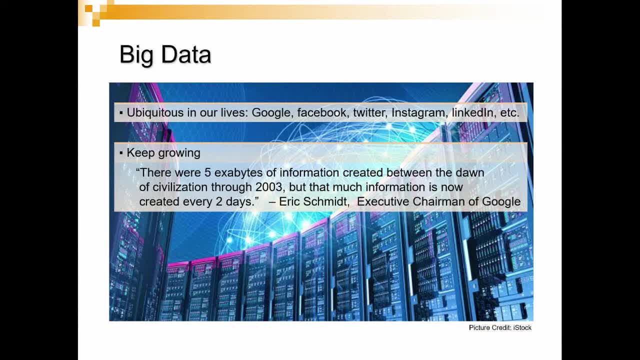 This is what he said a few years ago. There were 5x bytes of information created between the down Down of civilization through 2003.. But that much information is now created every two days. I think. I want to make two comments. 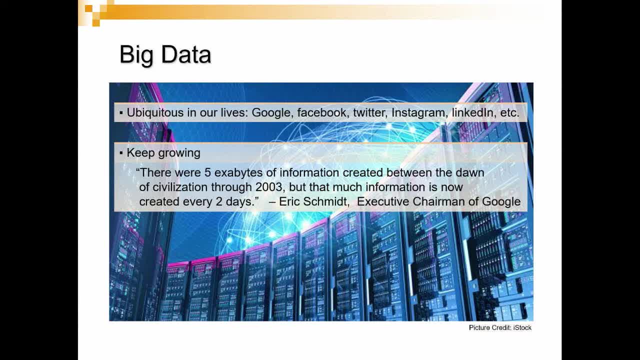 First of all, what is x bytes? X bytes is 10 to the 18th power, So that's billion, billion. Secondly, I think the word created probably is not the most accurate word. Probably should be recorded During the medieval times this information created. 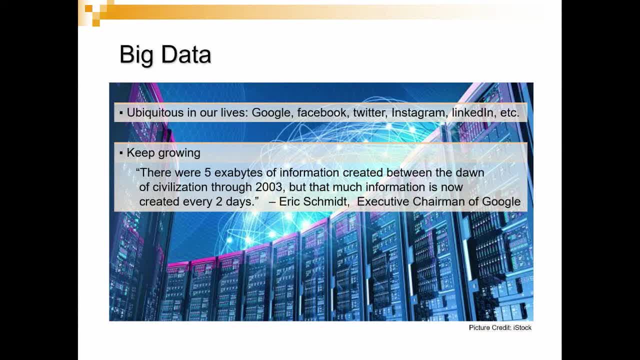 But they just don't have the means to record them. But now on Facebook, everything you did is recorded: You hate someone, You like someone. That's already recorded Already in the Facebook record, even if you decide 30 seconds later to delete it. 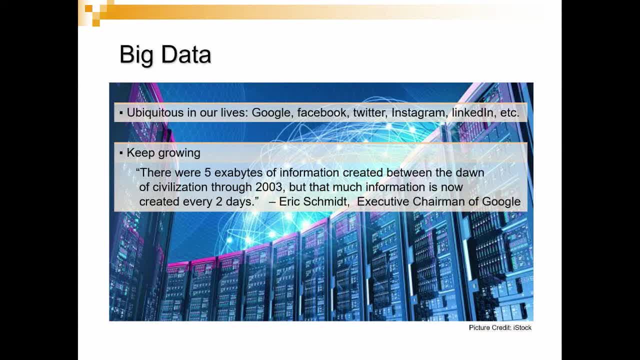 But then what you did before is already part of the official record, And this development, availability of big data and humongous amount of data create a lot of excitement, not only in the academic environment, like today, but also in government, industry and business. 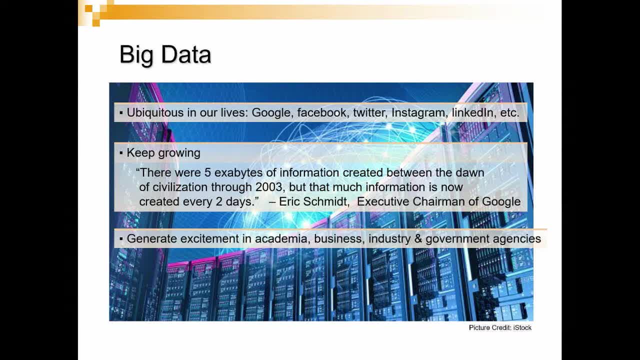 communities. As a matter of fact, if you go around talk about big data, you will realize that the vast majority of conversations of excitement or development about big data happens outside the academic world. For example, if you go to Wall Street, you'll find people talking about big data. 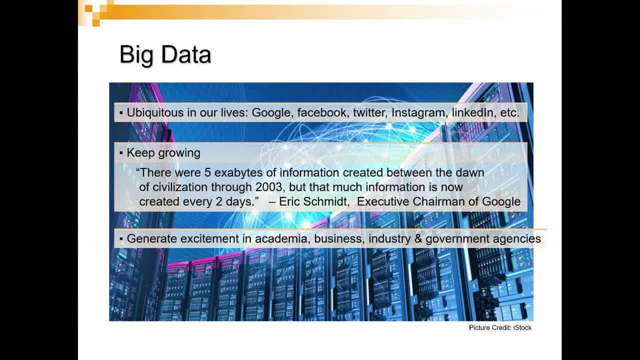 If you go to Silicon Valley, you'll hear people talk about big data. If you go to pharmaceutical industry, you'll hear people talk about big data. If you go to FDA, you'll hear people talk about big data. Even the CIA and FBI are talking about using big data. 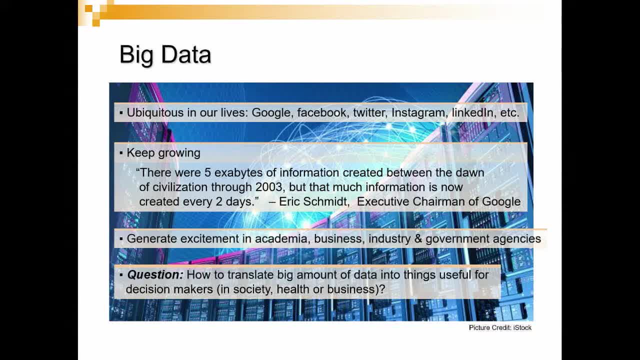 to catch terrorists and so on, And so, to a certain extent, I think for big data applications, the key question is that how do you translate such a huge amount of data into something that's useful for the decision making? That decision making can be decision making for business. 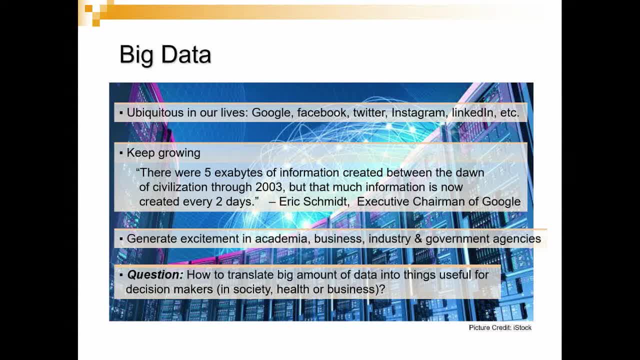 or decision making for the society, or the decision making from your doctors or health care providers to provide a better service, a better treatment for you. So in this talk we're going to look at big medical data. So here is a partial list of the availability. 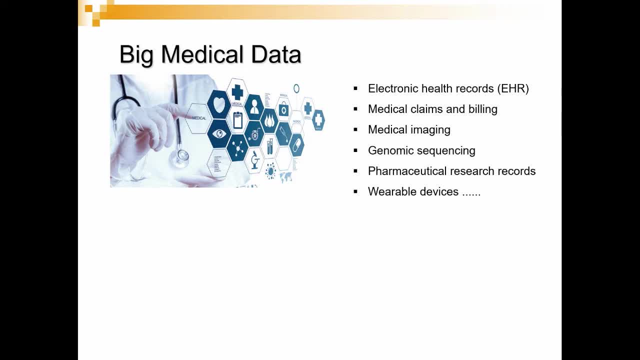 of different forms of big medical data. So let's go over them. First, electronic health record, And probably starting from 25 to 30 years, 25 or 20 years ago different hospitals and health care providers started to switch from the paper record. 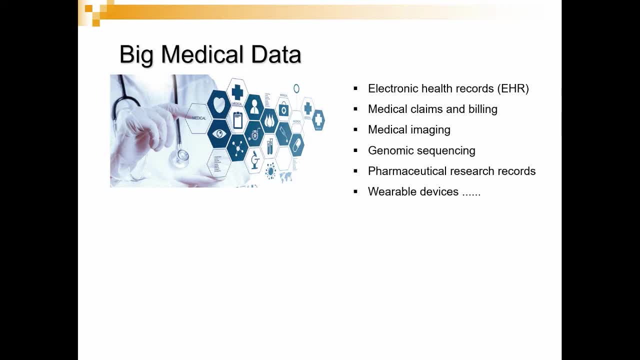 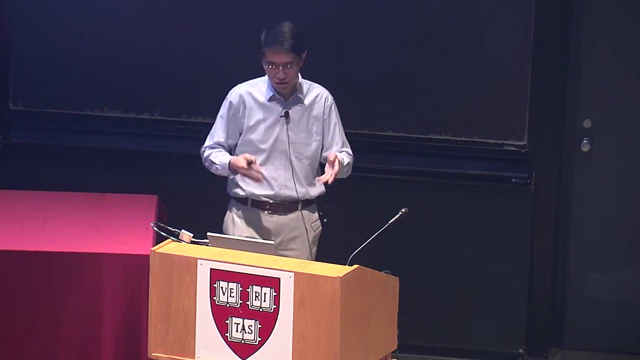 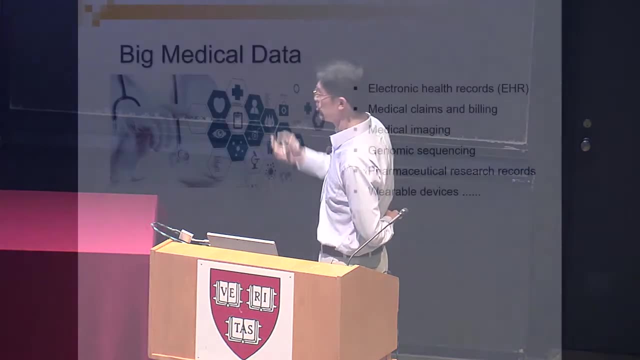 to electronic health record So that gives the doctors easy way to access data, enter your information, retrieve information and modify information. So that's the initial purpose, And so we have a huge amount of record of electronic health record. The second: why the huge data set? the insurance record. 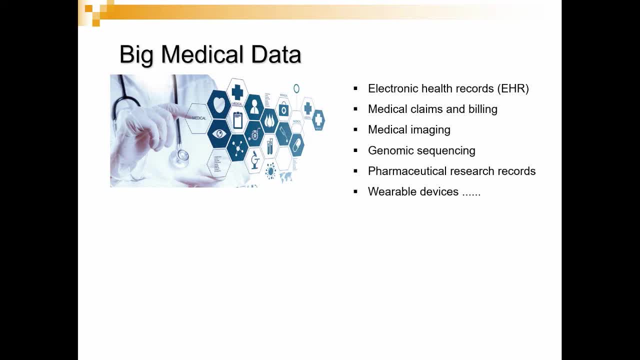 medical insurance record That mainly contains diagnosis, billing information for procedures, billing information for your pharmaceutical drugs taking, and so on, And so these two data sets are by far very large, And this data set actually, in a certain sense, complements each other. 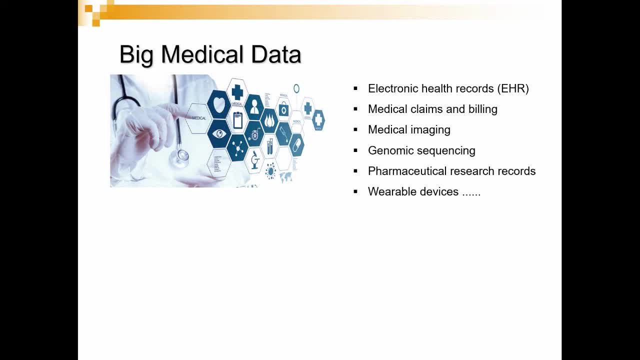 For the electronic health record. that's very granular. It not only contains the diagnosis but also contains the lab test And it also contains doctor's written notes. That is actually very useful information in many cases than just looking at the disease code and so on. 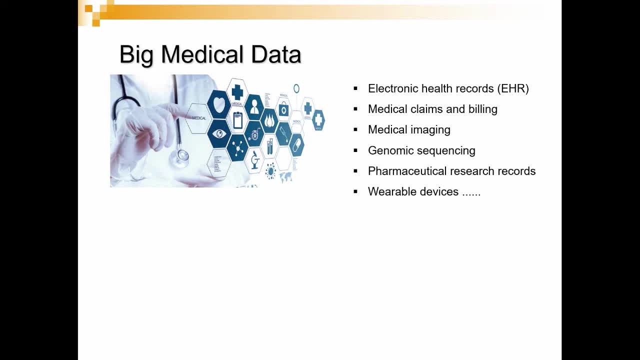 However, the electronic health record tend to be fragmented in the sense that, suppose you switch hospital from one to other. chances are that two hospitals are not linked together, So your data are fragmented, And that happens, for example, if you move your home. 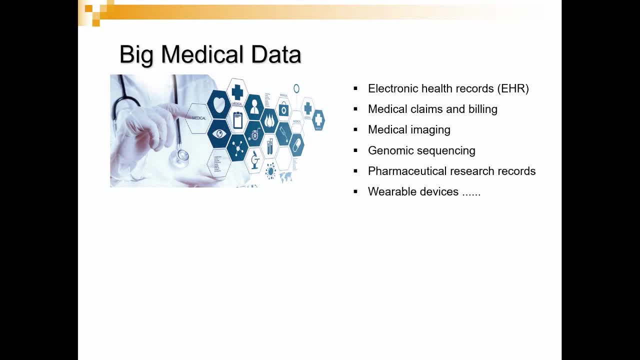 from one town to other. chances are you go to a different hospital health care provider And then your electronic health record are disjoint, the two pieces fragmented from each other Where the insurance record is not granular. the insurance record doesn't contain doctor's written notes. 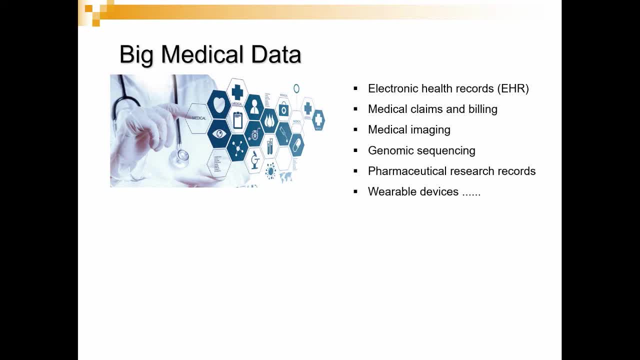 and so on. However, the insurance records are relatively complete, in the sense that, even if you switch hospitals, as long as you are under the same insurance plan, your health is actually reflected. And, of course, if you switch different insurance plans, things will change. 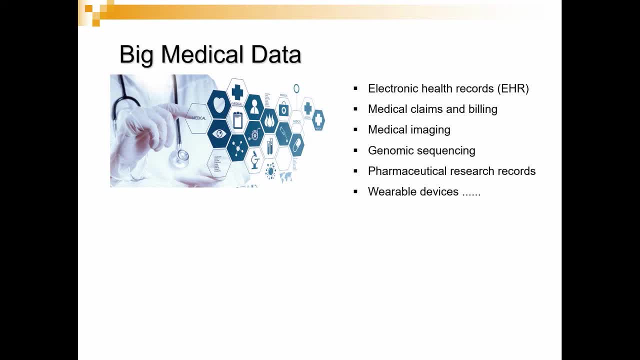 But chances are most of us we don't switch insurance plans that often. The biggest exception is that when people reach Medicare age 65 and so on, you switch to Medicare and Medicaid. That's one major switch. And so these are the two available large data. 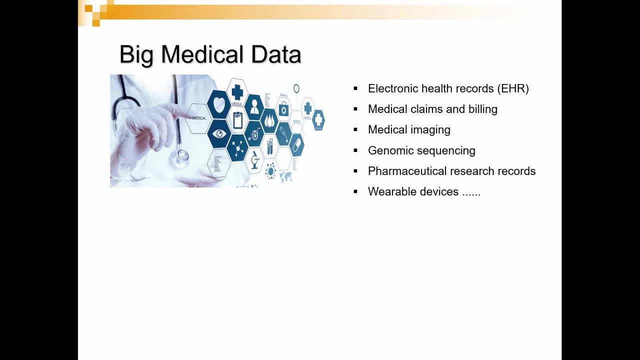 large medical data sets. The next one is medical imaging. In that case, we're talking about x-ray data, your CT scan data, your PET scan data and so on, And the size of medical imaging can easily go to terabytes and beyond. 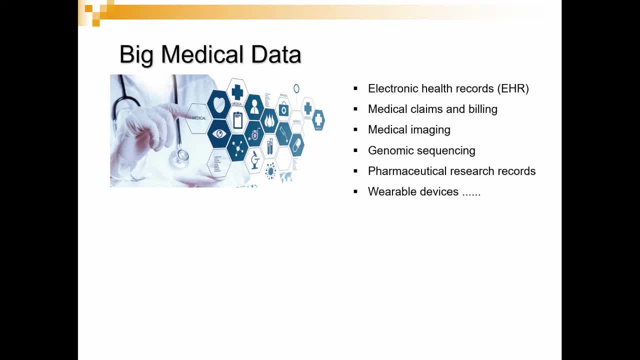 That's easy. And then that's genomic sequence data. The genomic data ranges from your test for single genes or a few genes or multiple genes, to a whole genome sequence, So that becomes more and more available for a lot of patients. Then there's the pharmaceutical research notes. 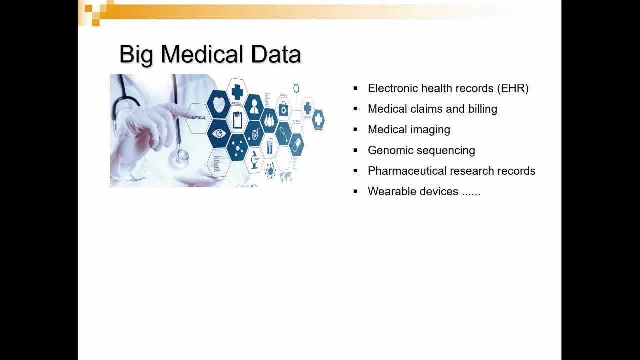 And those include the public available data. For example, there's a lot of publications, millions of publications at PubMed each year talking about associations between different chemical compounds or proteins to different disease conditions. That's one source of pharmaceutical record, And also in each of the pharmaceutical companies. 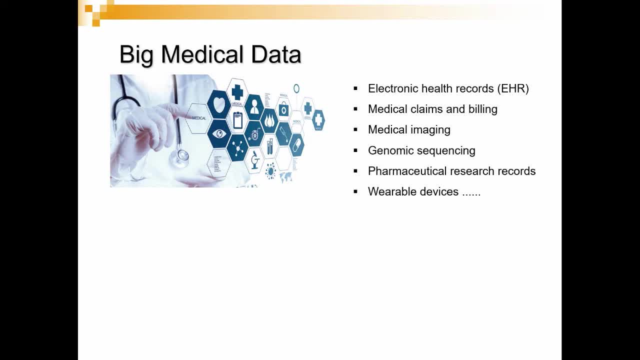 there's a lot of research notes left there in their database, But that's more like a private database. These are the available big data, big medical data. Then there comes the variable devices: the variable devices for Fitbit and so on. Not only tells you how many steps you work on. 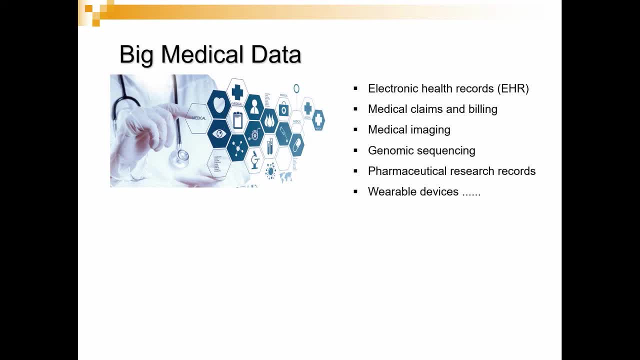 it also measures your blood pressure, measures your heartbeat and so on. Some of the medical devices, some of the wearable devices also, can accurately measure your blood sugar, But in real time. that also gives you a way to see whether your blood sugar 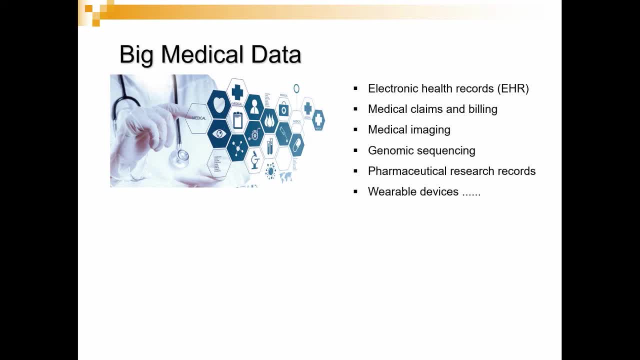 rises quickly after taking a risk: The rise of after taking bread, of after taking spaghetti, and so on. So that gives you fine control. And the wearable devices? now, some of the wearable devices actually also have some warning signal, for example, 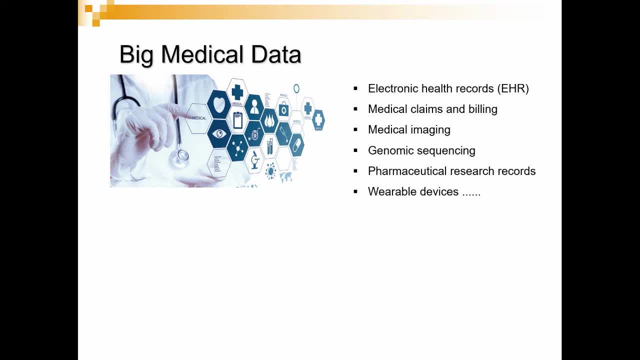 especially for older people. You see, you have a danger of falling, be careful, stuff like that. So the wearable devices become more and more available, nowadays prevalent, And all these available here is just a partial list. The list actually goes on and on and on. 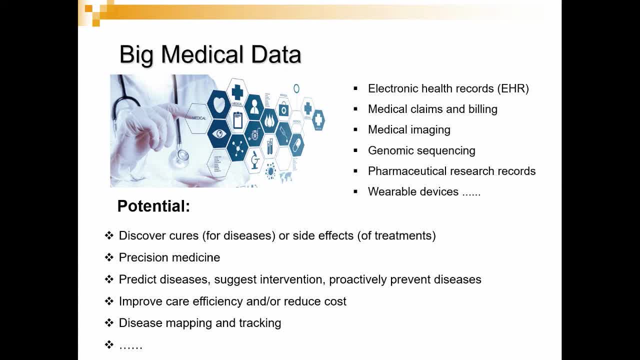 And all this opens up a lot of interesting potentials. So, for example, one potentials will be discovering new cures. For example, you're mining the pharmaceutical data sets, research record, you might find association, a very effective association between putting certain chemical compound and disease condition. 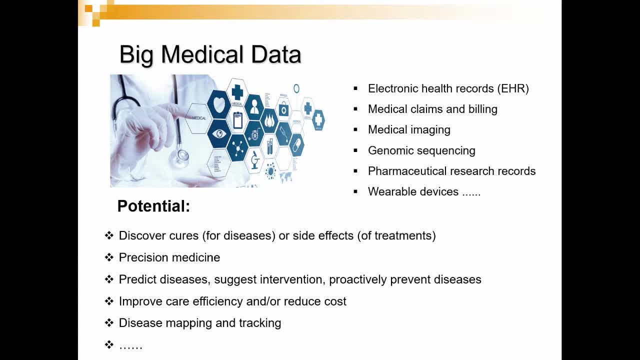 Maybe that leads to new drugs. Alternatively, if you mine the electronic health record or insurance record, chance that you might find that once in a while some treatment, some drugs designed from other conditions actually happens to be useful for other things as well. 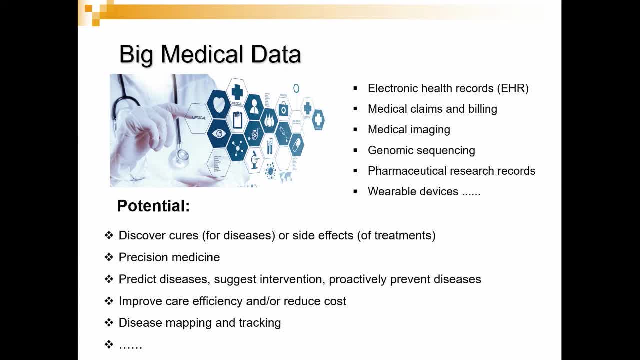 One concrete example would be Viagra, which previously was originally designed to treat a heart disease but later on it found useful for a different purpose. So that's one concrete example. Or you can find side effects of treatment, especially the emerging treatment, new treatment. 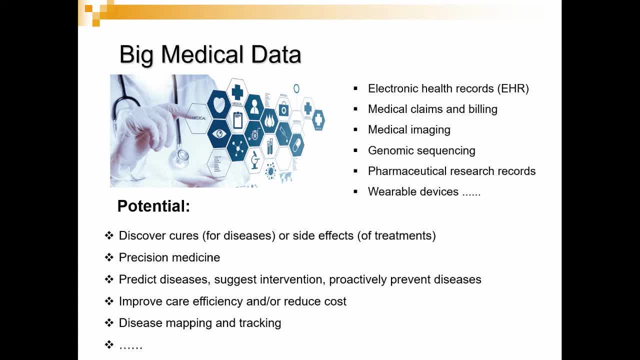 And then you can try to mine the data set, trying to find association, and try to find the causal relationship between the treatment versus the side effect. And then this opens the door of precision medicine in the sense that if you look at a patient past history- 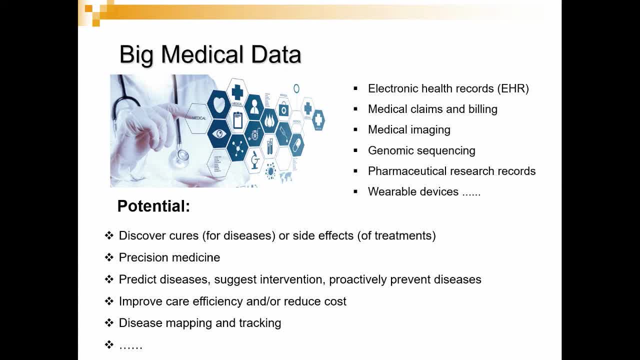 and disease history or health history, and maybe you can decide. for this condition, the best treatment is this rather than that. For example, two patients having the same, for example, skin disease, might have different treatment. One is giving you a steroid, the other give a. 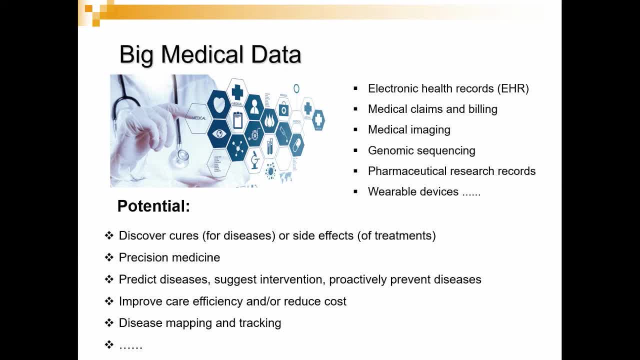 different medication to take and so on. So that's we're talking about precision medicine And also allows you to, potentially allows people to predict disease. Given the situation, maybe in the next six months something that's higher chance of this disease. 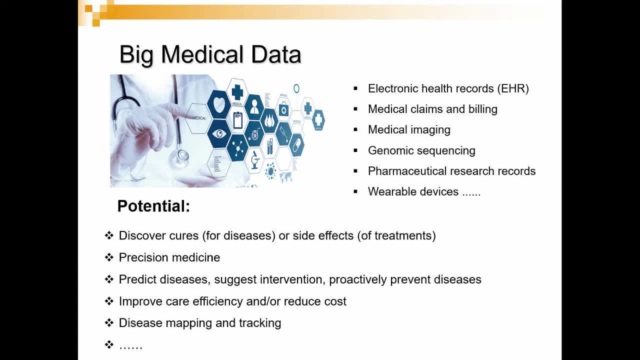 to develop for this patient, then you have to be careful. The doctors should notify the patient. the patient will take preventive actions And concretely, for example, support the patient that wants to do an open heart surgery and then, given the past history, there's a higher chance. 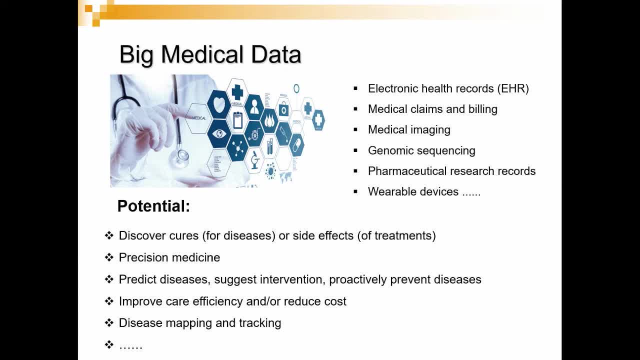 that major bleeding happens, Then probably before the treatment you should give, the doctors will give the patient some medications to alleviate the potential complication. And then also this all translate in the economic terms, translate to more efficient healthcare system potentially. 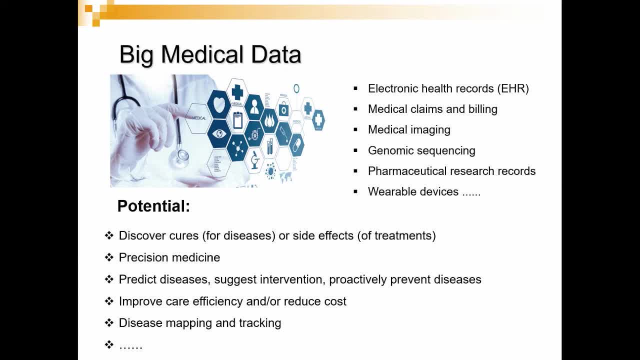 and reducing the cost for the healthcare providers as well for the patients. That's a big picture. And another thing: the combination of online platforms, social networks as well, for example, Google, Facebook and so on, as well as the electronic health record. 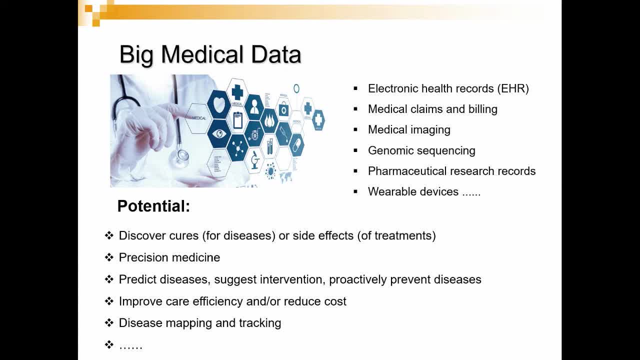 and insurance record give you a way to mapping diseases and predict infectious diseases. So in the past, in collaboration with many excellent coauthors, we work on mapping disease and tracking. Also, we work on mining the data set- PubMed public data set- to find associations. 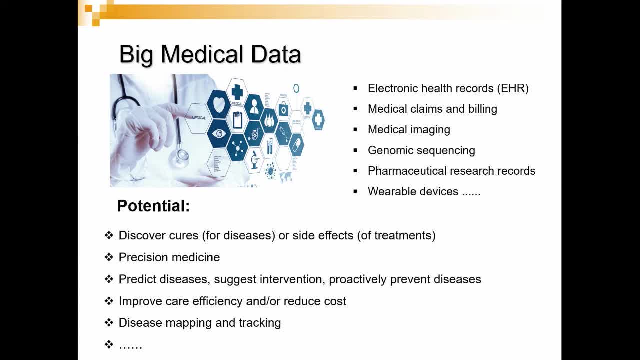 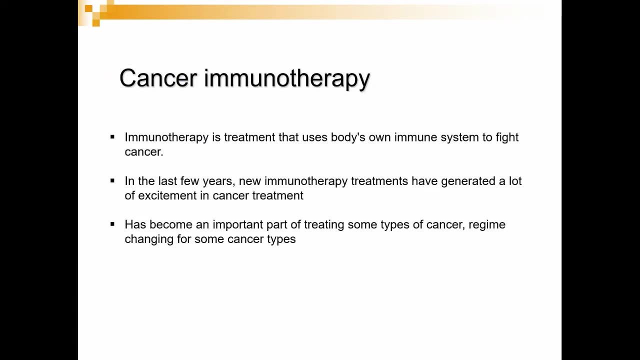 between different proteins and disease, But in today I'm gonna talk about the side effects of new treatment, emerging treatment and our discovery and our analysis. In particular, we're gonna talk about the side effects of cancer immunotherapy, And cancer immunotherapy is one of the. I think. 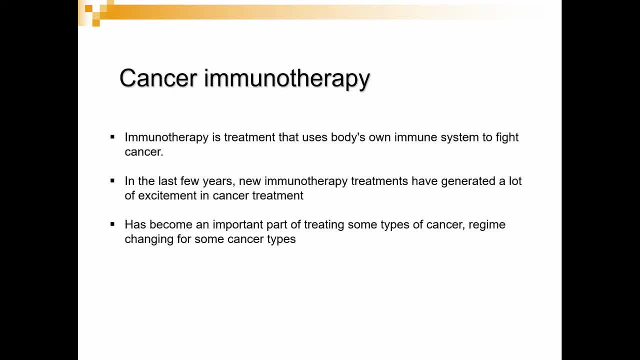 breakthroughs in the past three years And the first cancer immunotherapy drug approved by FDA is in 2014.. And later on, starting for 2015 and onwards, there's a lot more drugs approved by FDA for cancer immunotherapy. So the basic idea of immunotherapy sort of 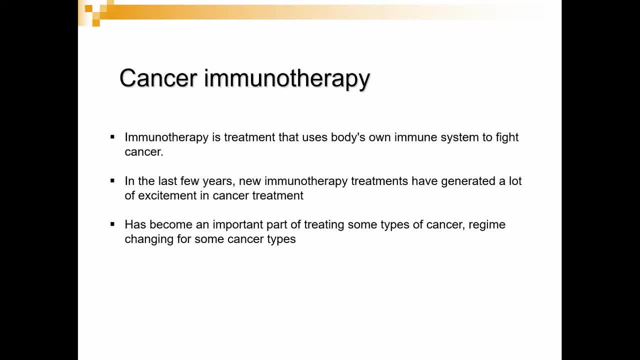 in certain sense is a regime changing for thinking about how to treat cancer. In the traditional people think about: let's design some compound to treat cancer. So you have to directly hit the cancer cell, directly to hit the cancer tumor. 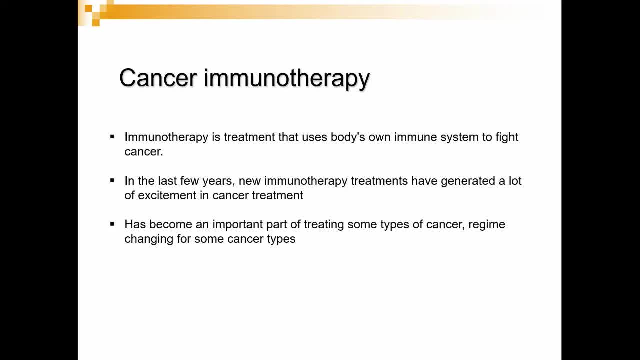 But immunotherapy turns the way around. It says: what if we try to tune up your immune system so that your immune system, T-cells and other things can directly attack cancer rather than through external compound? And so this has generated a lot of excitement. 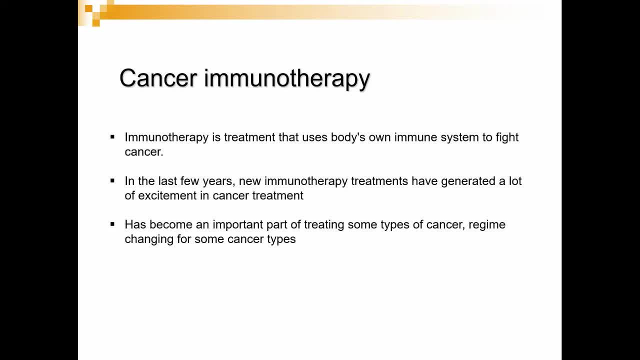 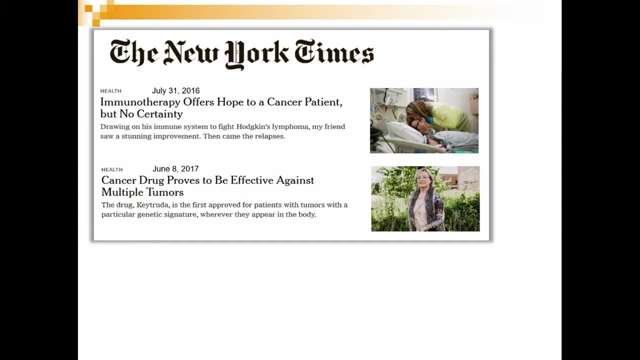 in the cancer treatment And, as I mentioned, it has become an important part of treating some certain types of cancer And in certain cases, that's a regime changing. People switch from chemotherapy to immunotherapy, you can see, And this, of course, not only generated excitement. 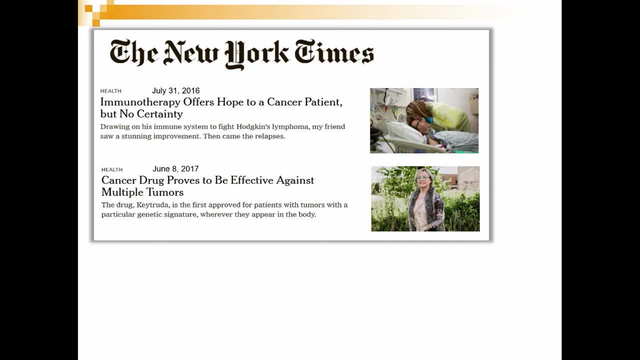 by the doctors and so on, oncologists. it's also generated a lot of excitement in the public media And eventually, actually if you Google in all the public media, you'll find some articles here or there discussing about immunotherapy. 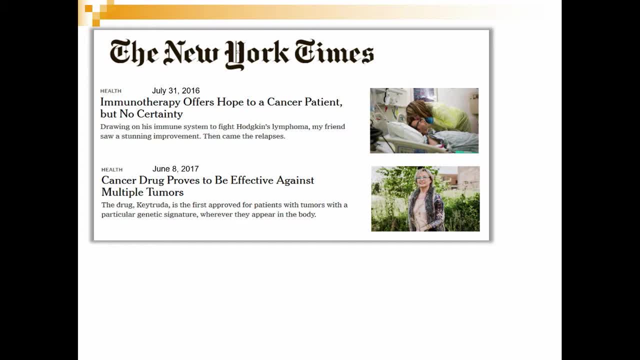 So here are two articles from New York Times and you can see I won't read the details, but basically say cancer immunotherapy offers hope and provides a very interesting result, and so on. Here's from Wall Street Journal. Also talk about cancer immunotherapy treatment. 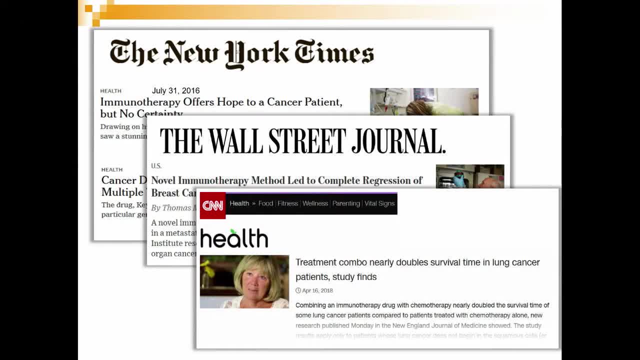 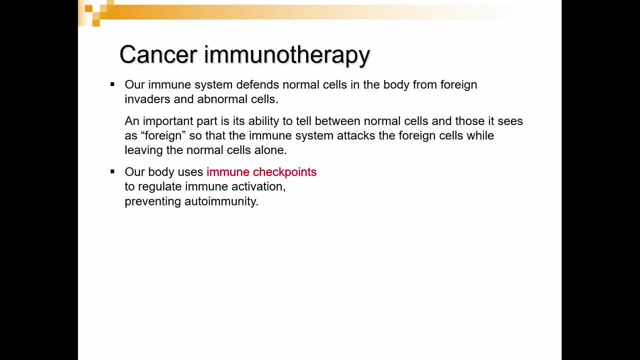 for breast cancer, And here's the CNN. Cancer immunotherapy provides remarkable treatment for lung cancer patients, and so on, And so okay. so before I talk about the side effect, before I talk about our analysis about the undesired consequences of immunotherapy, 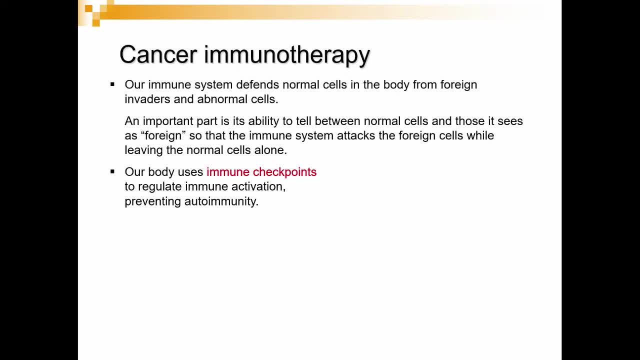 let's first talk, spend a few words, talk about the specific cancer immunotherapy that we're gonna looking at. Just we can now we have to start from our own immune system, because we are using immunotherapy, using our own immune system, to fight cancer. 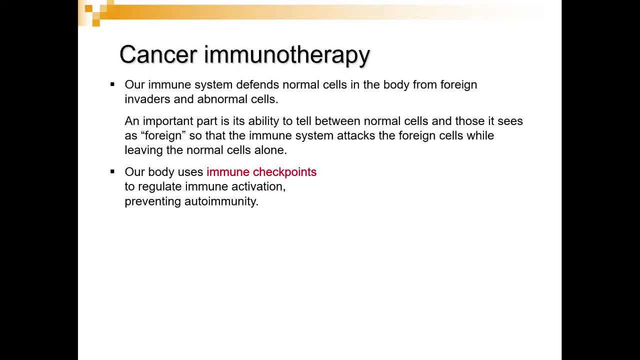 The immune. our one important part of immune system is to defend our normal cell from the invaders- virus, fungus or bacteria- And as well as abnormal cells, And so a crucial part is for immune system to recognize who is the bad guy, who is the good guy. 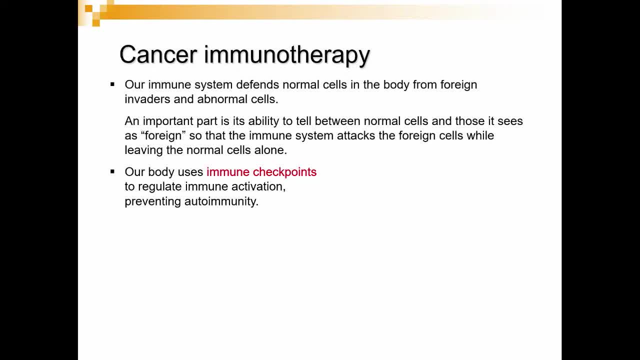 So the immune system should leave the normal cells alone and start concentrating, attacking the invaders or abnormal cells. okay, One mechanism for our body to regulate the immune response to avoid onset of autoimmune disease, which is the case that immune cell, your own immune cells, start to attack normal bodies. 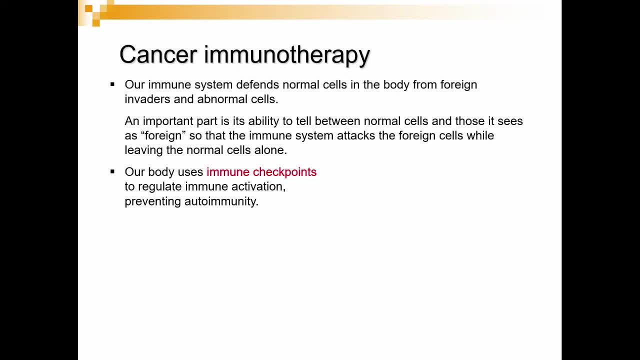 that's autoimmune disease. To avoid this development of autoimmune disease is so-called immune checkpoint. So one of the important immune checkpoint is so-called PD-1, PD-L1 checkpoint. So here's the diagram. So let's talk about normal cell. 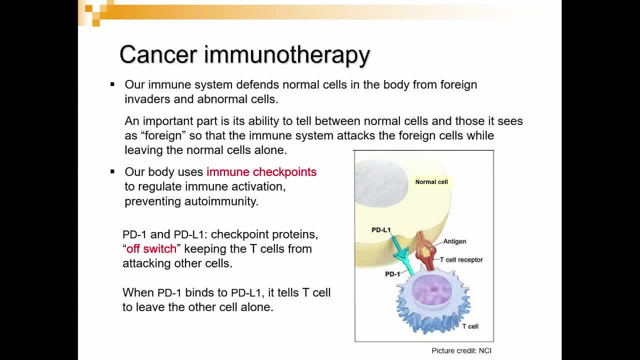 In normal cell. it very often happens that in normal cell, on the cell membrane that's a lot of antigens, So this antigens attract T-cell to bind to them. However, for our own body, in order to avoid the T-cells to attack the normal cells, 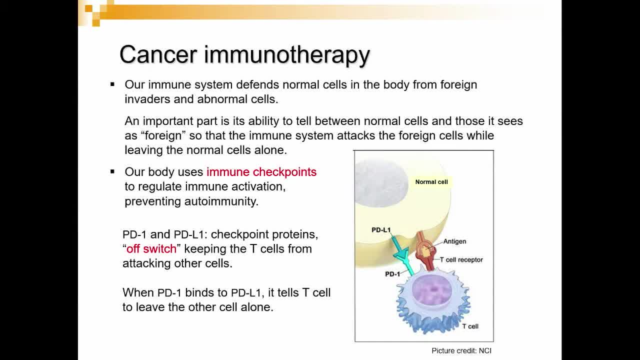 there's some pathway, so-called PD-1 and PD-L1 pathway, And the PD-1 is a protein that binds to the membrane of T-cell And PD-L1 is a counterpart, binds to the membrane of the normal cell. So when the PD-L1 and PD-1 binds to each other, 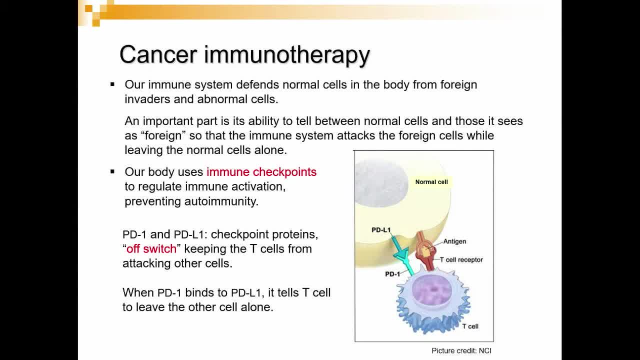 it signals to the T-cell that this is a good guy, this is our own guy, so leave it alone, go away. So when the binding of PD-1 and PD-L1 happens, it essentially deactivates the T-cell. 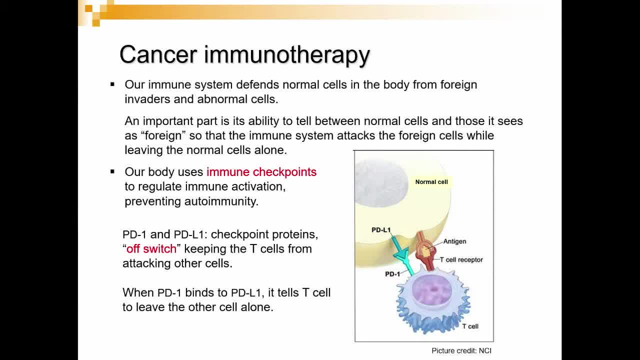 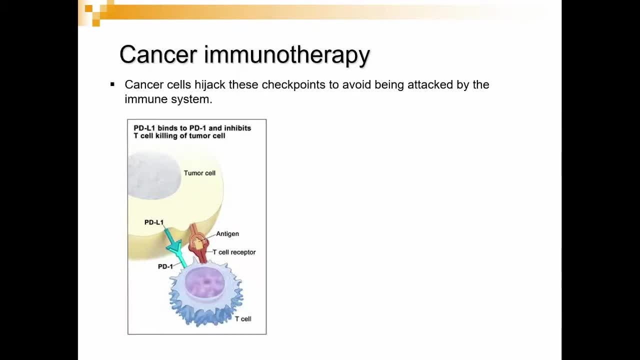 so the T-cell goes away won't attack the normal cell. So that's one of the ways our immune system tries to regulate our immune response. Unfortunately, the same way our immune system regulate to tune down T-cell is also hijacked by many cancer cells. 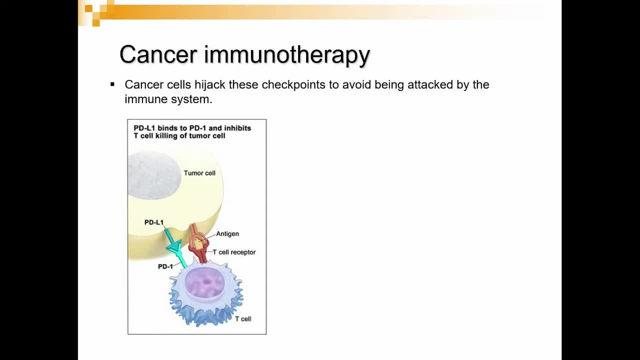 In many, many cancer cells. there are lots of PD-L1 proteins on the surface of a cancer cell. So the cancer cell: because there's a lot of PD-L1s, it binds to PD-1 and then send a false signal to the T-cell. 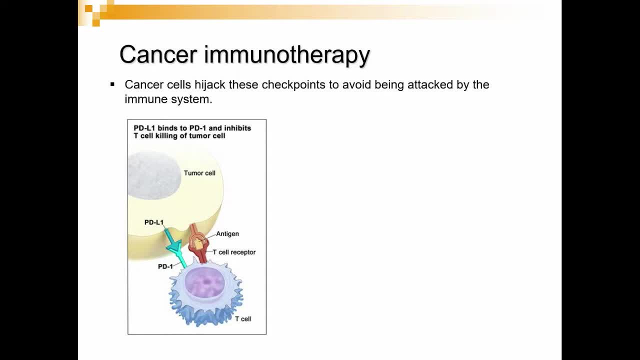 this is a good guy and don't do much damage, go away, And so that's a way, one of the major ways for the cancer cell to avoid being attacked by T-cell. So that generates the idea of checkpoint inhibitor. 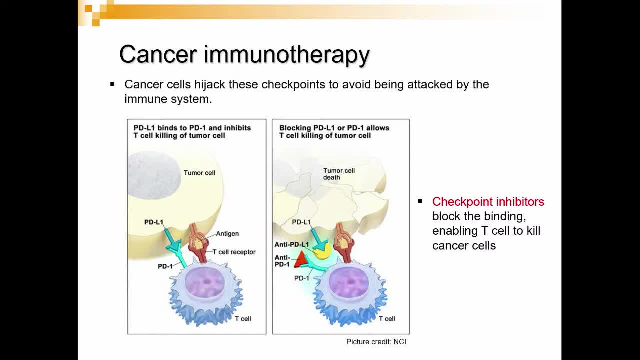 where there are the small proteins designed to bind with either PD-1 or PD-L1.. Once they bind to PD-1 or PD-L1, they prevent the binding of PD-L1 and PD-L1, and so that blocks the signal pathway. 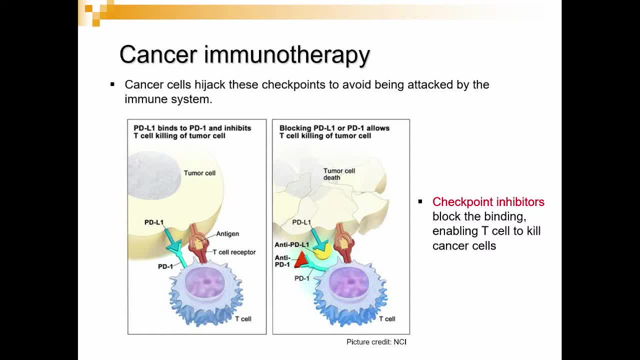 for the cancer cell to send the false signal to our T-cell So that enables T-cell to start to attack tumor cells, start to kill the tumor cells. So that's a basic idea of checkpoint inhibitor. This idea later on developed to a lot of blockbuster commercial drugs. 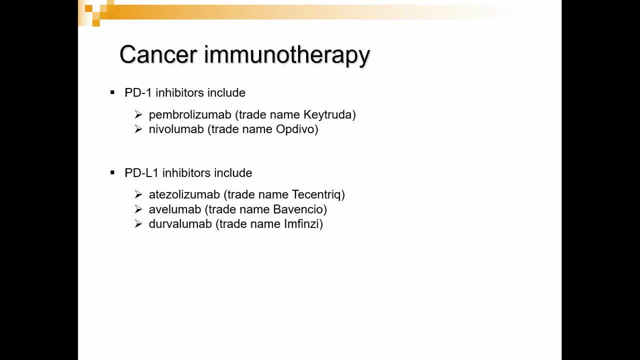 For example, right now in the market there's a lot of these are the drugs partial list of the drugs approved by FDA- Either block PD-1 or blocks PD-L1. And by far these two are the most prevalent drugs. 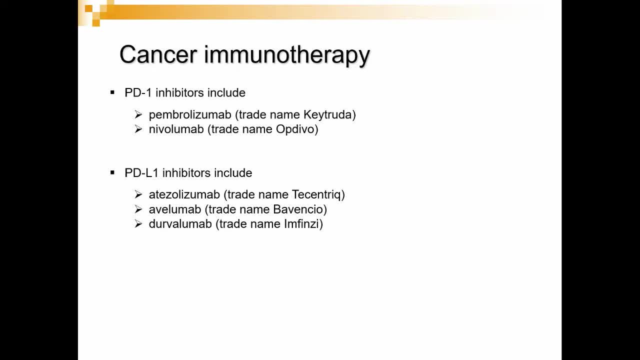 And they're under the name Pembrolizumab, Nivolumab and so on, And you'll notice that this name is difficult to pronounce. but many other drug companies have trade names over them. For example, The treatment for pembrolizumab is Keytruda. 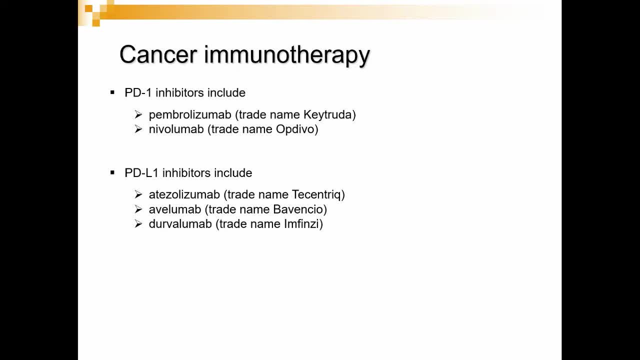 The treatment name for nivolumab is Opdivo, and so on. Keytruda is a billion-dollar drug for Merck. So now, each year it generates a billion-dollar revenue for Merck. Okay, so now what we're looking at now. 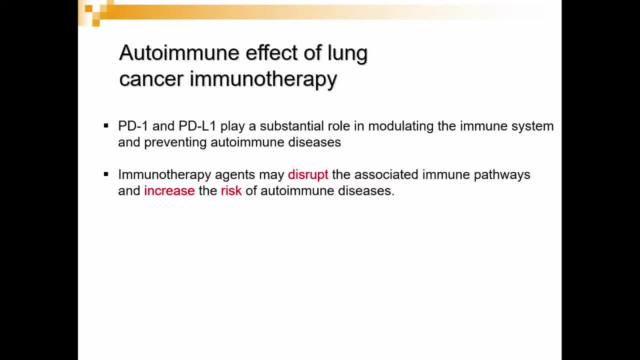 are the undesirable consequences of immunotherapy. And the intuition is actually relatively straightforward, Since PD-1, PD-L1 is an important part of our body to regulate immune system to prevent autoimmune diseases. Now you interrupt the pathway, Chances are you might disrupt the normal regulation of immune response. 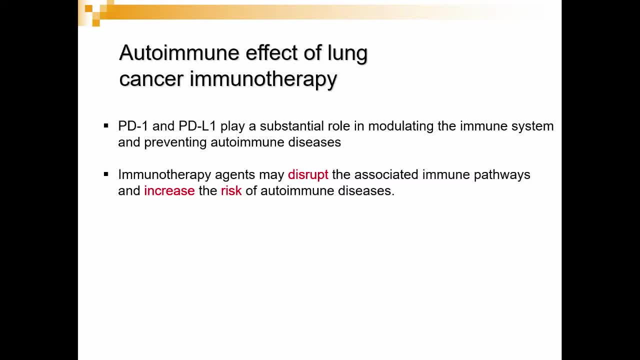 and that might lead to autoimmune disease. You block the binding in cancer cells. Chances are you also have to block the binding of normal cells And in fact the onset of autoimmune disease has been reported by doctors, but in more anecdotal lines. 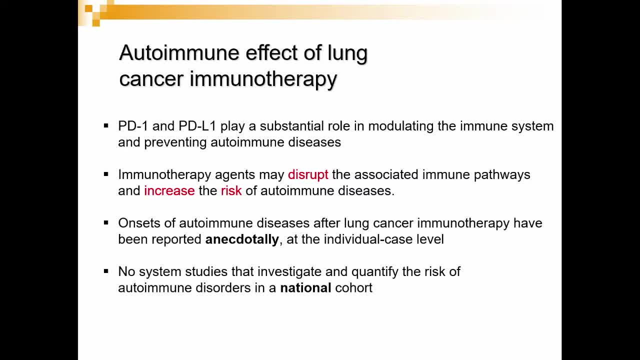 it's been reported that there's been a decrease in the incidence of autoimmune disease. So far, as far as we know, there's no population study or there's no systematic studies to study to address the effect of the undesired autoimmune effect for cancer immunotherapy treatment. 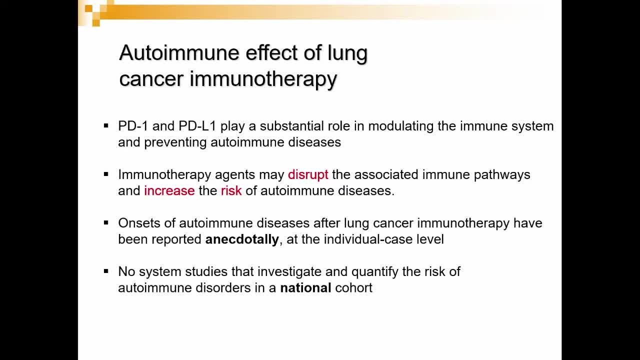 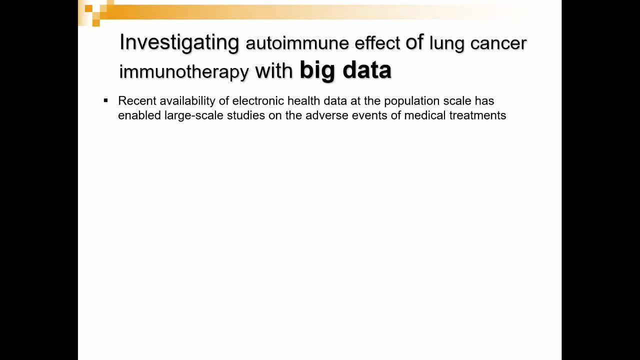 So that's where we start with And we're talking about, especially at the national cohort. there's no such study available. So in our case, well, the reason- availability of big electron houses, data at the population level- enables the large-scale study for a situation like this. 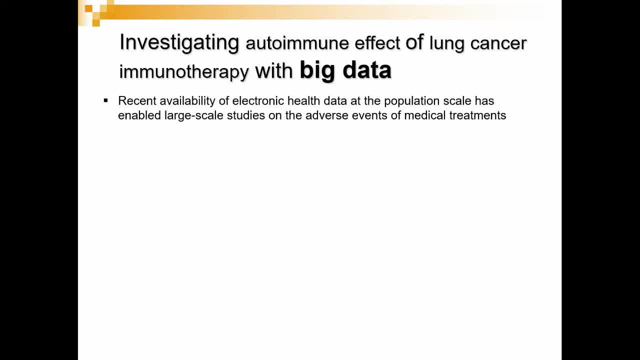 and to study especially rare or emerging treatment. medical treatment In our case, available to us is our de-identified national insurance cohort that covers 44 million members in the United States, And the insurance data provides a diagnosis code and procedure That includes pediatric treatment and pharmaceutical treatment. 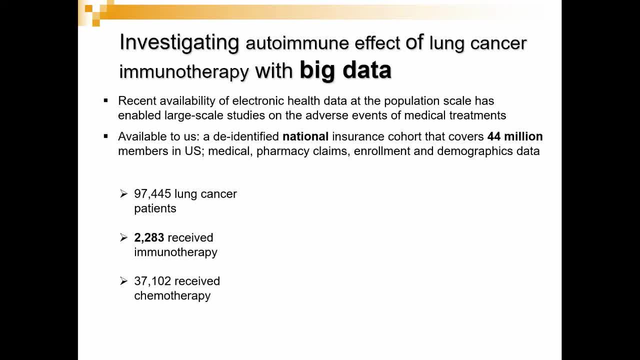 and so on: pharmaceutical prescription and so on. It also includes the patient's zip code, for example, and demographics and enrollment and so on. So out of this 44 million member record, there are roughly 97,000 lung cancer patients. 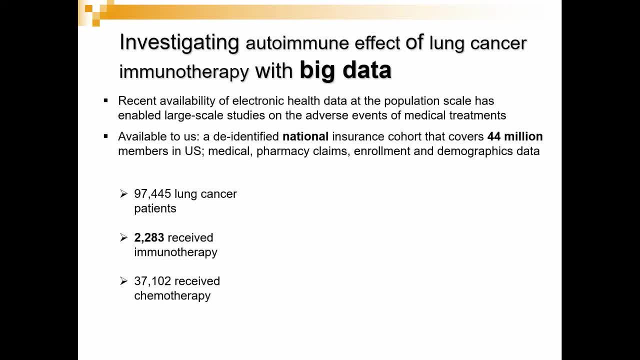 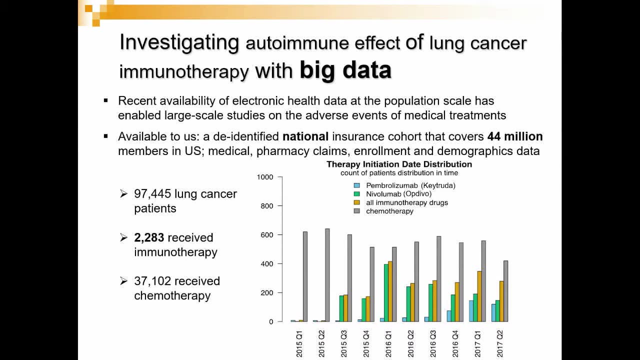 And among them roughly a little bit over 2,000 patients have received immunotherapy and another 37,000 received chemotherapy. So this picture illustrates what's going on. Remember, the first immunotherapy drug, PD-1, L1, is approved in late. 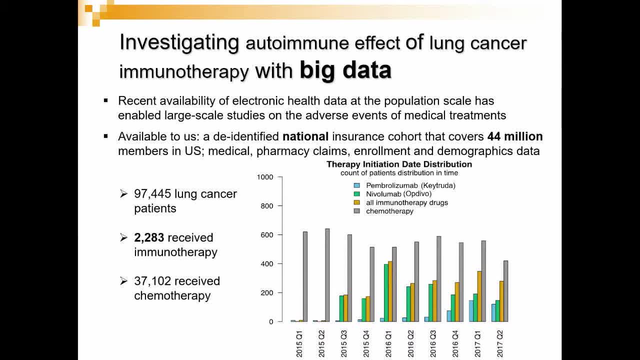 2014 and now this picture shows the arrival of the cancer immunotherapy treatment. the gray bar is chemotherapy- pretty much stable before and fluctuate, now started going down. and the yellow bar is all immunotherapy you treatment in this database and the green bar and blue bar are 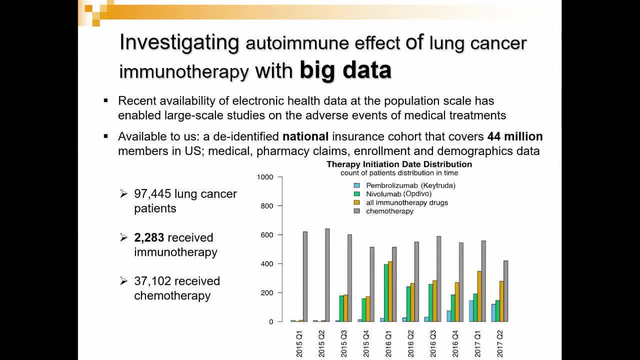 the two dominant immunotherapy drugs: Kituda is the blue one for, and green one is Optebol. It's interesting that you see from this picture all the又 퍼ты start to see a regime change Before 2015,. pretty much everybody is on. 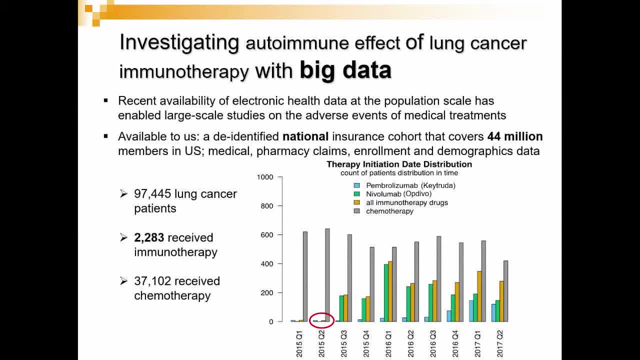 chemotherapy. There's only less than 50 patients receiving immunotherapy, But as you go onward you realize that the total immunotherapy started to become on par with chemotherapy. As a matter of fact, right now it's roughly 50-50 if you keep on going for 2018.. So you see a 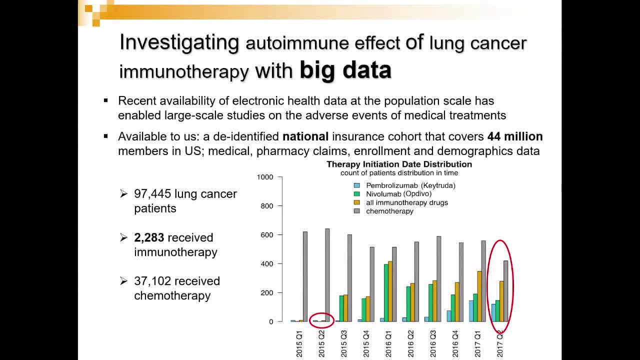 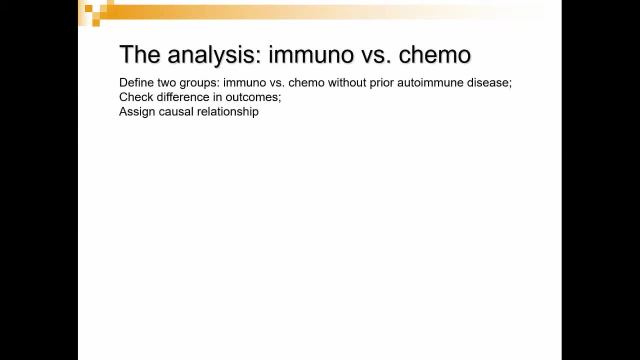 regime, changing of lung cancer treatment. And now, in this case, we're studying. we're trying to study the effect of immunotherapy, the autoimmune undesired consequences of immunotherapy. So, naturally, what do you do? Well, now you have two groups of populations, It seems sort of the rest of the story will be. 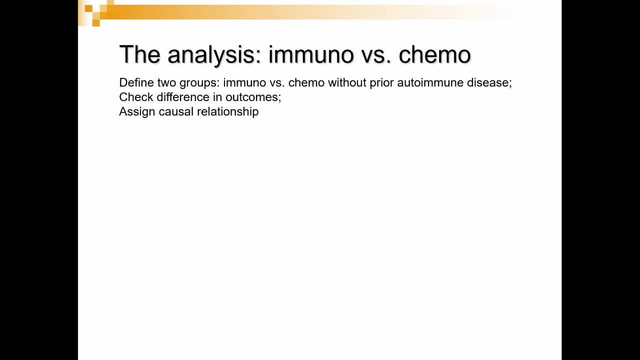 straightforward. We have two groups of patients: immunotherapy patients versus chemotherapy patients. Well, we check the difference in the main outcomes From the initial treatment initialization. how long does it take them to develop autoimmune disease? for patients who might never develop autoimmune disease, Then that's the 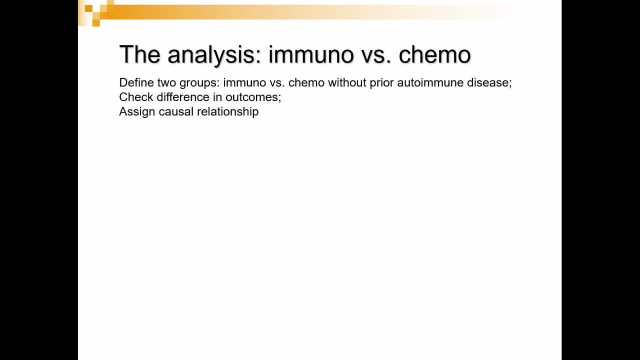 sensor data, And it might take the patient three months to develop autoimmune disease and so on, So naturally. and then you can assign causal relationship. That sounds like a very natural thing to do And, as a matter of fact, you can even do plot, calculate p-values and so on. So this plot shows this is so. 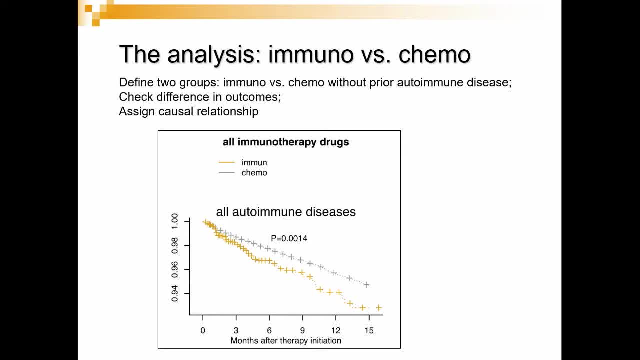 called the Kaplan-Meier curve, the probability of a patient not having autoimmune disease three months, for example, six months- after the initial initialization of the treatment. And the fact is that if you look at the curve, the chemotherapy curve is above the autoimmune, autoimmune immunotherapy curve. 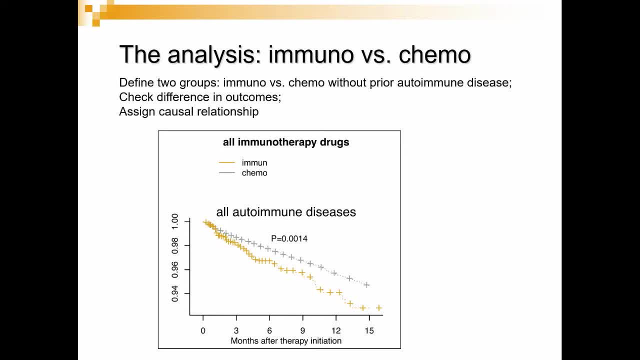 That basically tells us that fewer patients from the chemotherapy treatment are reporting onset of autoimmune disease compared with the immunotherapy disease. As a matter of fact, you can also calculate the p-values using based on Kaplan-Meier curve and so on. Does this not sound typical or sound similar? As a matter of fact, in a lot of 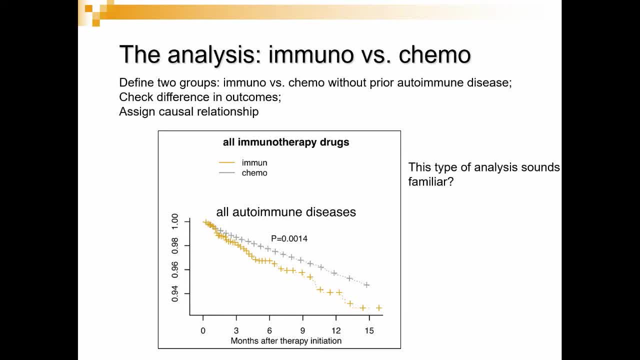 medical analysis, you encounter a picture like this Survival curve, Kaplan-Meier curve. then they calculate p-values. But I have to say this is naive at best. Even if you can calculate p-values, that's actually naive at best. 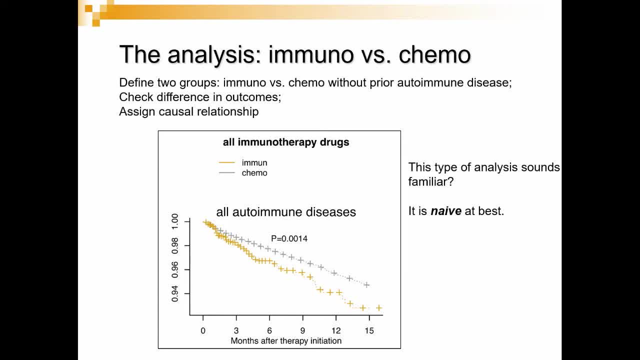 Because fundamentally we're talking about the causal relationship. We're arguing that immunotherapy might or may not lead to cause more autoimmune disease. We're talking about causal relationship. So, to illustrate what is going on, what's wrong with this type of analysis? let's take an extreme case. Let's take a 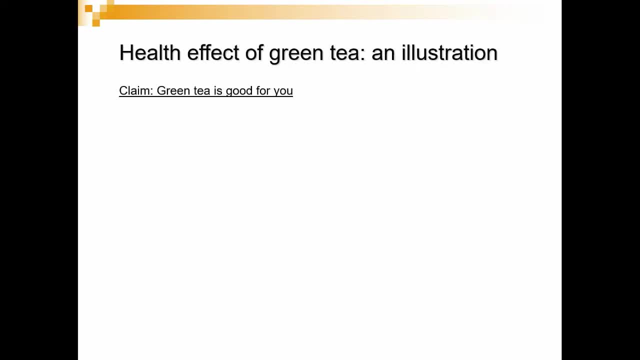 kind of case talk about. let's take a hypothetical case. Let's see the health care effect of green tea. Okay, Green tea is good for you. In this case you can back up. you can even back up this with some. 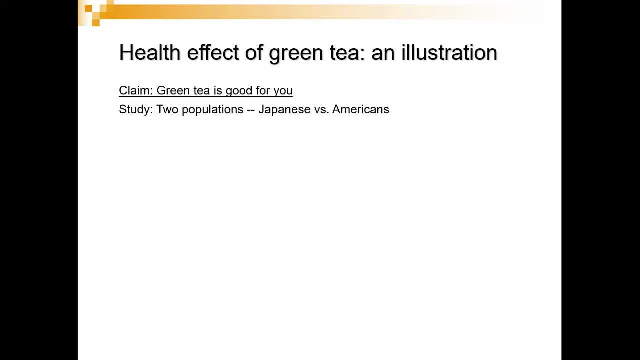 data, For example, two populations, the Japanese versus the Americans. Japanese drinks a lot more tea than Americans Green tea and they are the observation: the Japanese have much higher life expectancy than Americans and overall cancer rate is much lower in the Japanese population. I think I've reversed, order this to the numbers. 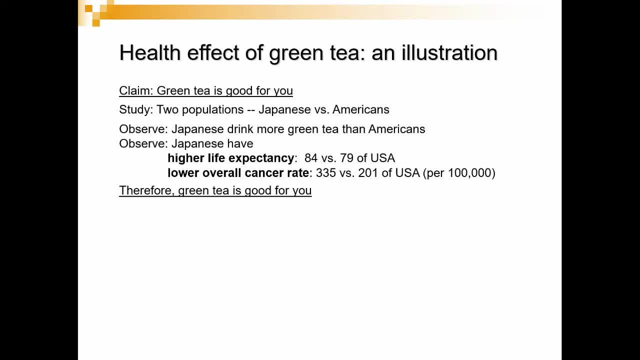 should be reversed: 201 versus 335, I accidentally typo- and therefore green is good for you. as a matter of fact, you can back up with if you want. you can back up survival curves and so even calculate p-value to justify this. but what went wrong with this analysis? well, first what went wrong, what I would say. 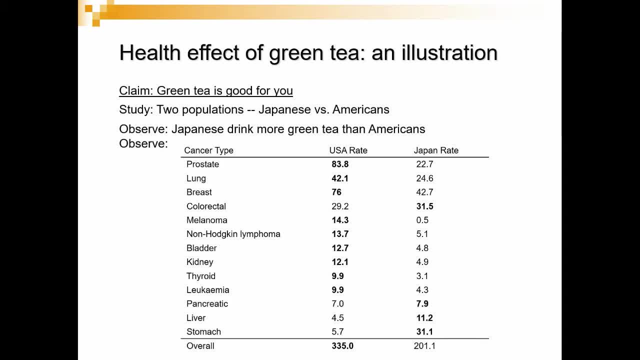 this is not naive at best. first went wrong is that we have all cancer types. now let's zoom in for a lot of the cancers. indeed, US rate is higher than the Japanese rate, but it's not so. if you look at liver cancer, Japanese case is twice more likely to develop liver cancer. 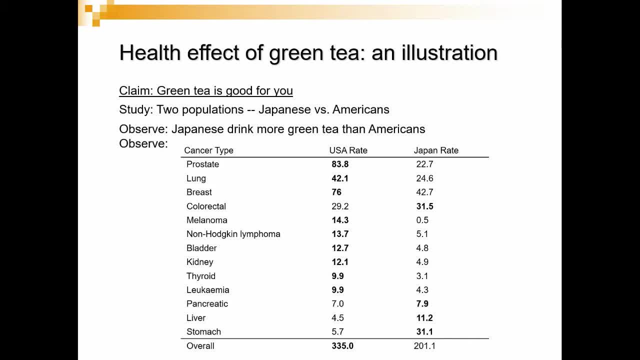 for stomach, it's five times as high. well, now I start questioning. green tea, something after you swallow to your stomach. now you have a high problem: stomach cancer. doesn't this really mean this, might you believe, more than skin cancer, for example? okay, what's going on? well, that's only the part of iceberg. the 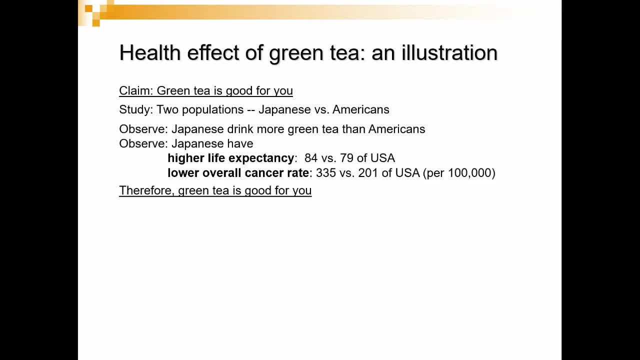 fundamental question is that. the fundamental question is that I can stop. I can stop you to stop the green tea by a lot of other things, for example, sushi. the Japanese eat a lot more sushi than Americans and but they have a lot higher expectancy, lower cancer rate. therefore, sushi is good for. 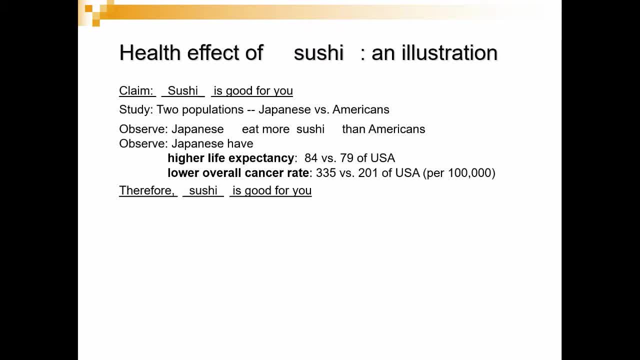 you, you can argue for the same thing. so, fundamentally, the underlying problem for for this type of argument, for this type of calculation or this type of p-value calculation to justify whatever is there, is because this two populations- they are trying to talk about treatment versus control- the two population fundamental. 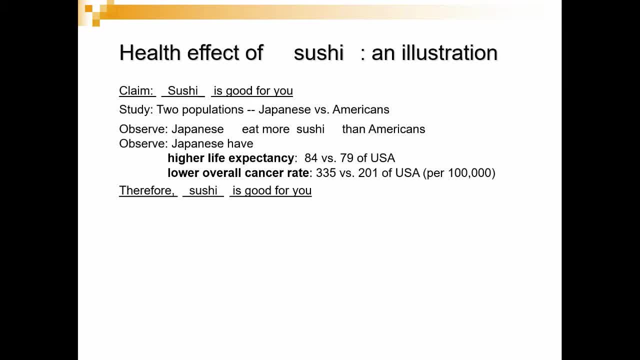 different, the environment is different, the lifestyle is different, the family structure is different, the diet is different, the genetics are different. so you can't there's tons of hundreds of millions of difference you can talk about. therefore, in this case, that actually no way you can assign causal. 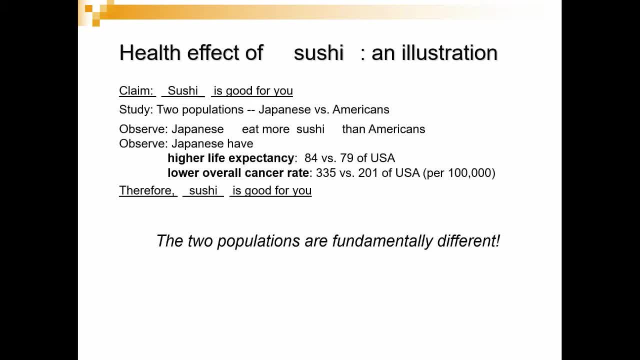 relationship, but unfortunately you know a lot of pop, pop cultures in other medias. we see this type of analysis all the time for something you might say: tomato is good for you. why tomato is good for you? look at a small village in Italy. well, people eat a lot of tomatoes. they have had people, happy people. 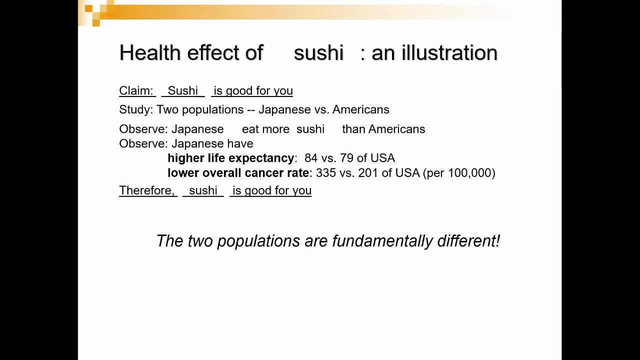 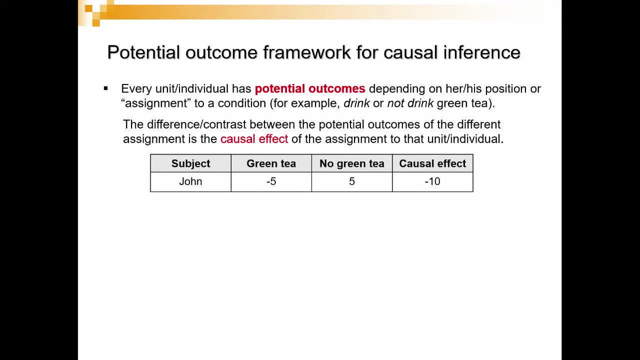 have like low cancer rate and so therefore tomato is good for you. but this type of analysis is this type of story see a lot from medias, so you know my opinion. the right way to think about causal inference is really the potential outcome framework. so here's a basic idea. so every unit has a potential outcome. on 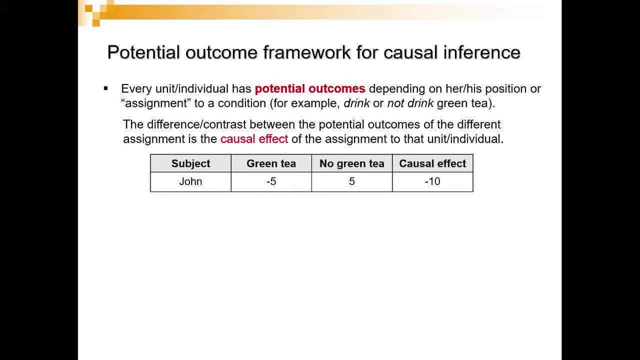 the different condition on the assignment: assignment for the conditions, for example. here's a concrete example: John taking green tea or versus not taking green tea. taking green tea, three months later, you find John's blood pressure was lower down by five points, whereas if John don't take green tea three months later, his 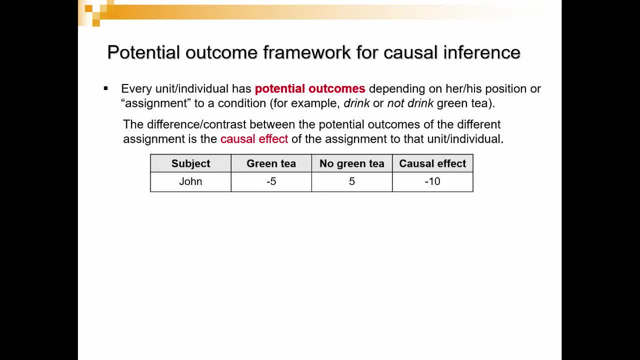 blood pressure increased by five points, then we see the difference. 10 is drinking green tea. in John's case, he can lower his blood pressure by 10 points. so the difference or contrast between John's potential outcome under the two different conditions, that is what we can contribute as a causal. 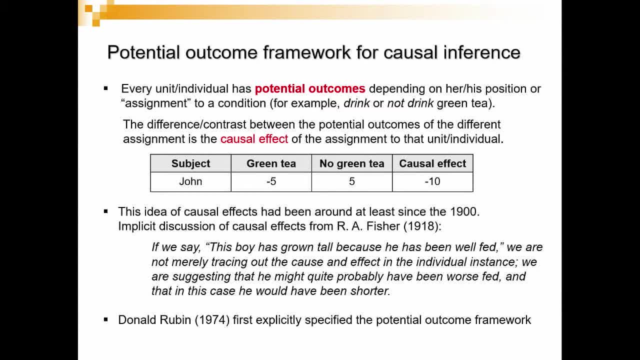 jer of this particular condition and this idea looks like a very transparent ly. it has a relatively short history compared with the whole history of science and this round, this idea, has been around since the 1900, for example, RFisher, the founding father of modern statistics and founding father of modern theory of genetics. this is what 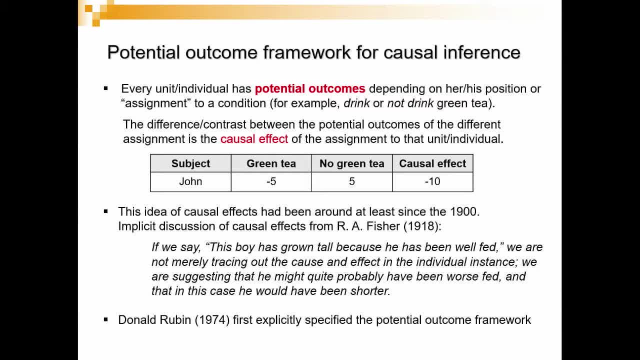 he said implicitly what he wrote implicitly, talking about this type of causal effects, back in 1918.. This is what he said: If we say this boy has grown tall because being well-fed, we're not merely tracing out the cause, the effect in the individual instance. 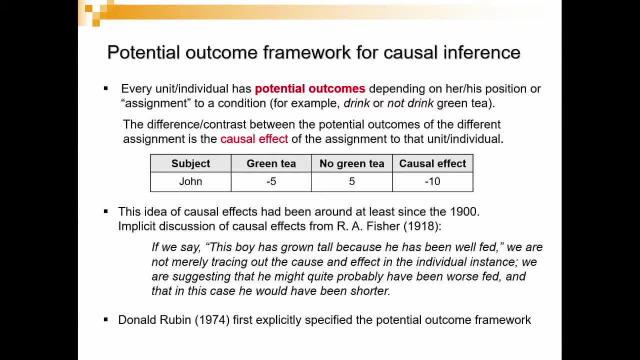 we're suggesting that he might quite probably have been worse fed and that in this case he would have been shorter. So you see that Ari Fisher back in 1918 is already talking about potential outcome If this boy is well-fed versus not well-fed. 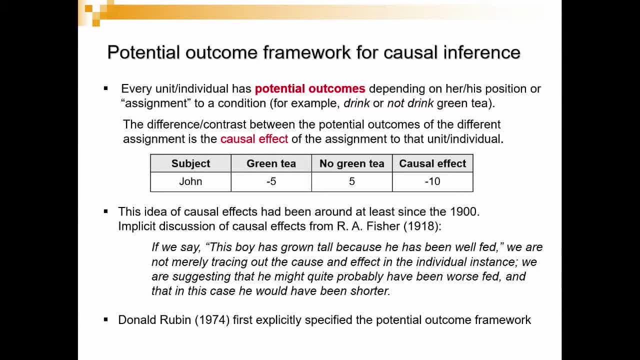 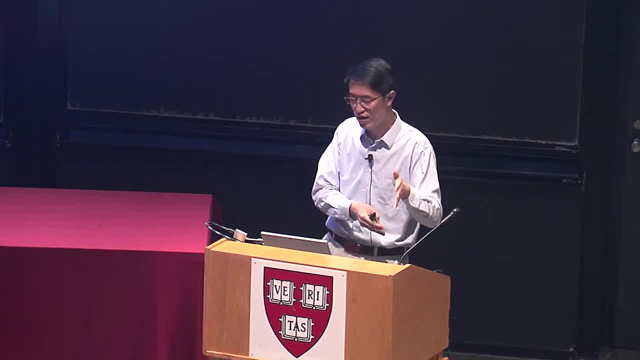 then if we trace the difference years in the future, then we can assign whether his height and so on is grossing his height to the initial condition, that is, he's well-fed or not well-fed. But history has to wait until 1974.. 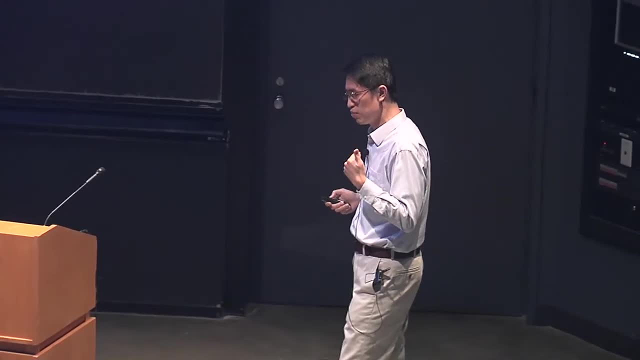 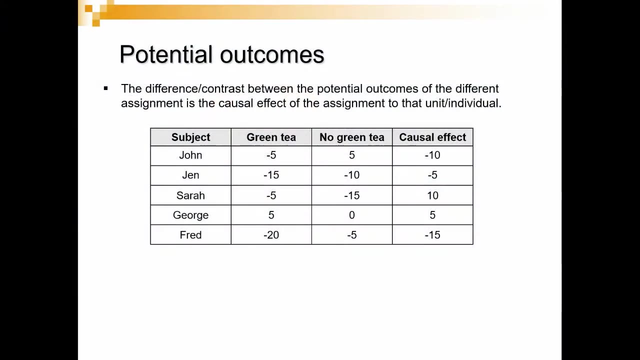 Don Rubin, my colleague at Harvard State Department, the first person to explicitly specify this potential outcome framework. And so, to put it in a nutshell, we'll talk about causal effect for individual. Now we have a population, We can talk about causal effect for the population. 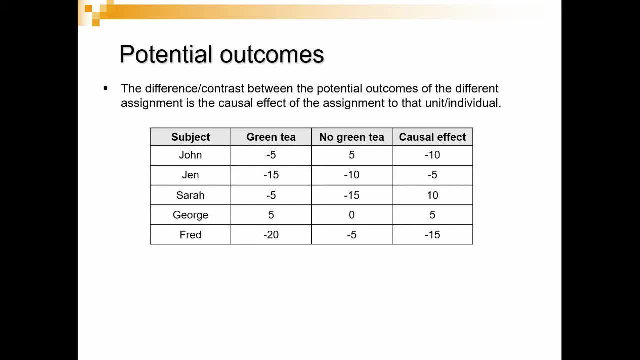 For example, John. the causal effect for John taking green tea is to minus his blood pressure by 10 points. The causal effect for George, who is taking green tea, is actually not very good for George. He increases his blood pressure by five points, and so on. 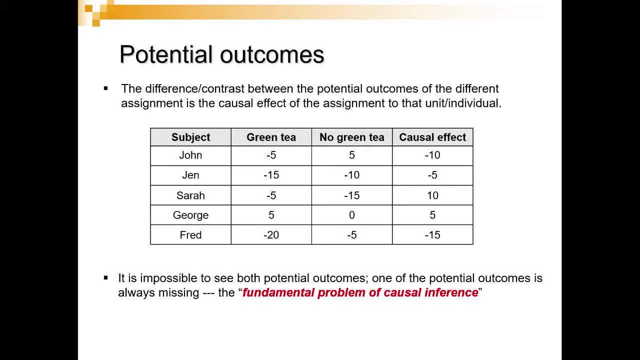 But then we encounter the fundamental problem of causal inference, That is, in reality, we only observe one arm: John is drinking green tea. We don't observe what's going on if John is not drinking green tea. In other words, we cannot go back to time. 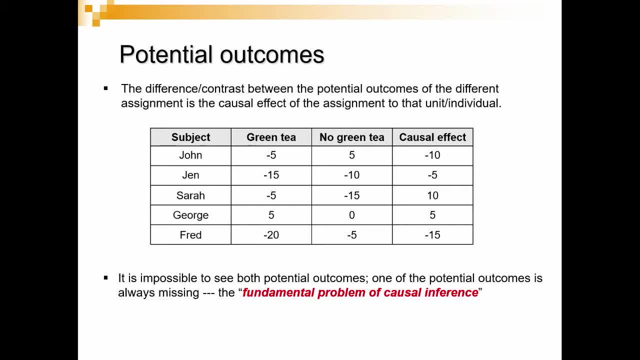 and watch the parallel universe. We only have one universe, We only have one time: evolution. We don't have that. Then that creates. so at least half of the data is missing on this causal inference framework. So what do you do? Well, one of the most profound ideas. 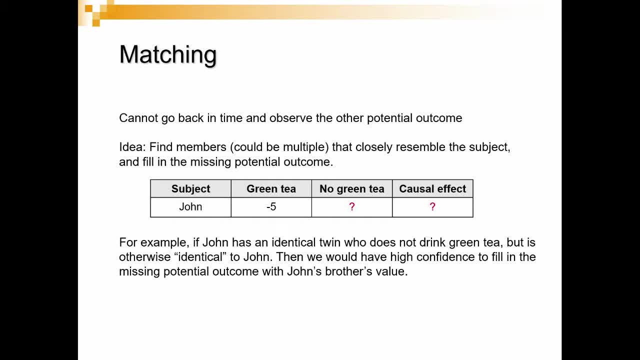 of tackling this problem is to match it. We cannot go back to time. However, if we can find a member or multiple members in the control arm that matches John to a large extent, then we can use their value to substitute for the missing value. 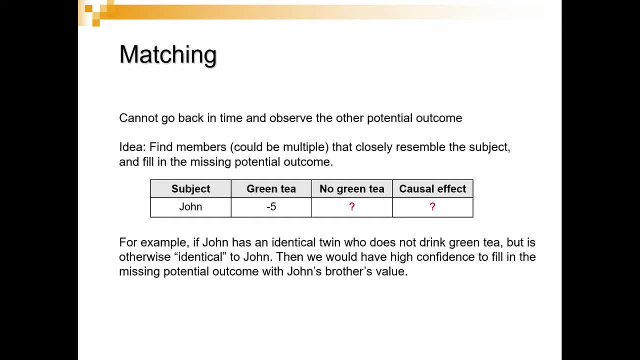 that we're looking after. For example, supposing that in an extreme case John has an identical twin who looks otherwise like John in every aspect, except this identical twin is not drinking green tea, Then we can attribute the effect. We can reasonably convert the field. 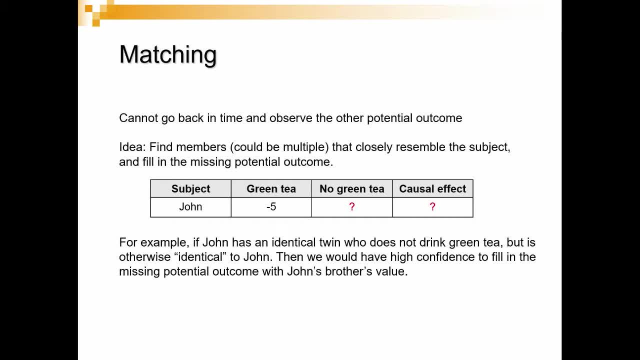 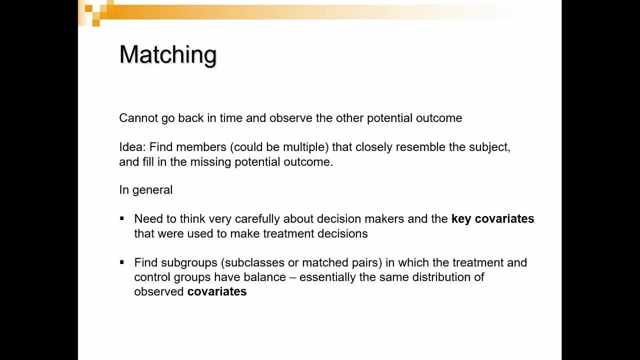 this number to John's case under not drinking green tea. Well, in reality, we're not that lucky. We don't have an identical twin situation. In reality, we need to think in order to fill the missing data using matching. we have to think very carefully about decision makers. 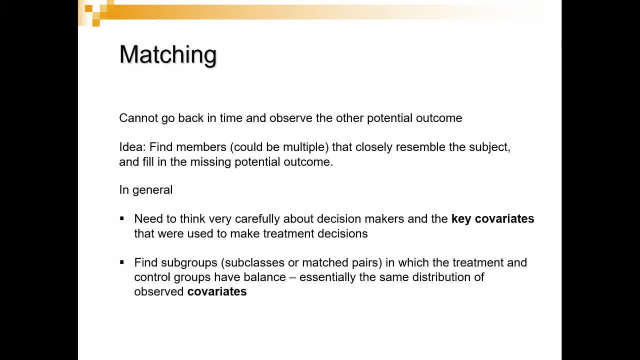 and what are the key covariates that we use to make treatment decisions, And then we try to find subgroups in which the treatment and the control groups have good balance. By good balance we mean essentially the balance of all the important observed covariates. 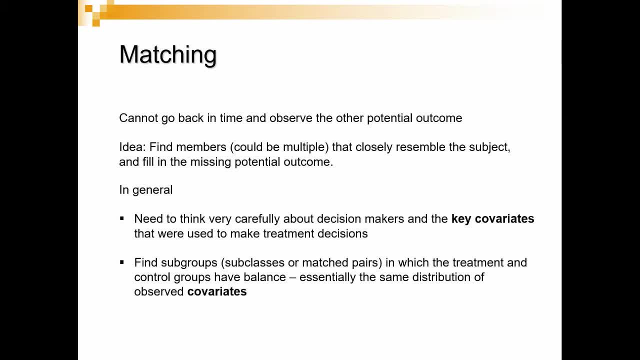 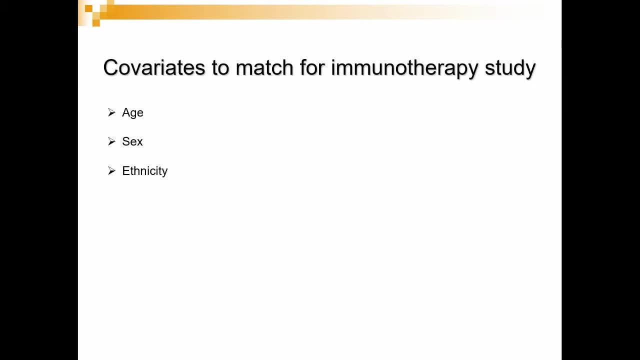 Then we can try to study the causal relationship. We can use the potential outcome to study the relationship. Okay, Now let's get back to the immunotherapy study. What are the important covariates in this case? Well, we talk about oncologists. 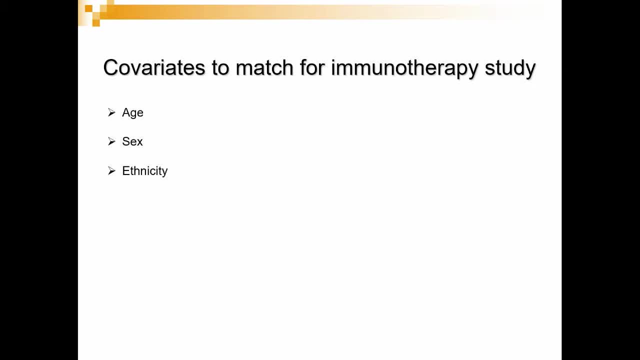 Some of the obvious important covariates are the age, sex and ethnicity. That's sort of obvious And young people and old people respond, potentially respond differently, And different genetic makeup respond differently. But also social economic status is important. 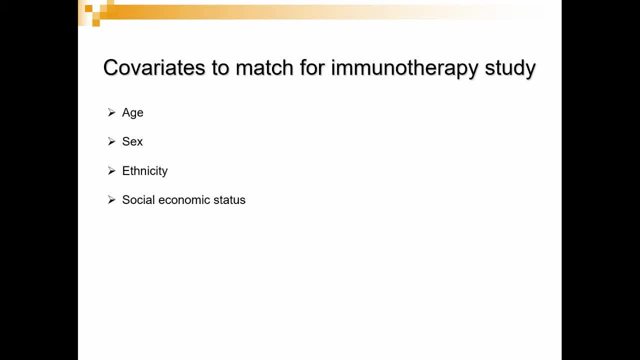 The wealth. the wealthy people and the low-income people respond differently because their lifestyle is different. They want the control for that And we don't have a social economic status. but we do have the median income of each zip code and the median unemployment rate in each zip code. 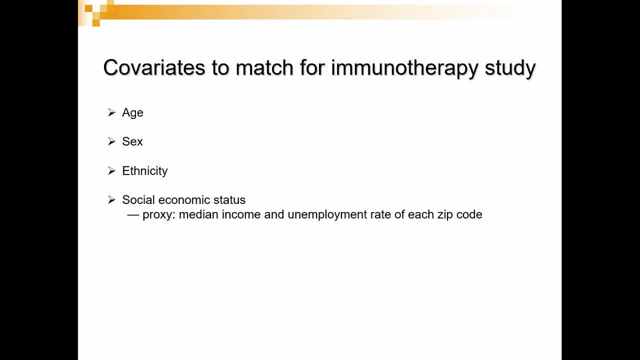 That's from US Census. We can use that information as a proxy for social economic status, because for each member we have their zip code: Healthcare utilization. Some people are more health conscious, Whatever disease they have, whatever condition they have. 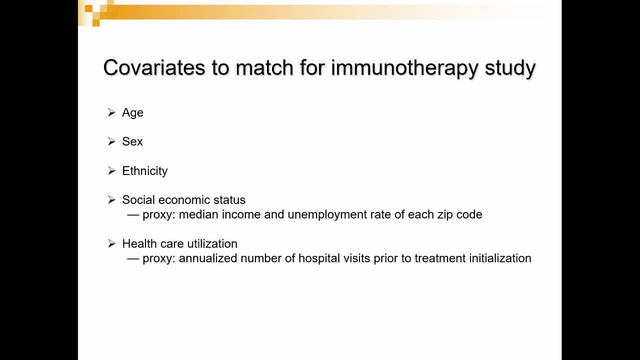 they go check the hospital. Some people don't want to go to hospital. Maybe they go to hospital every 10 years or something. So these two people, this type of group of people, you don't want to match each other. You want to be very careful. 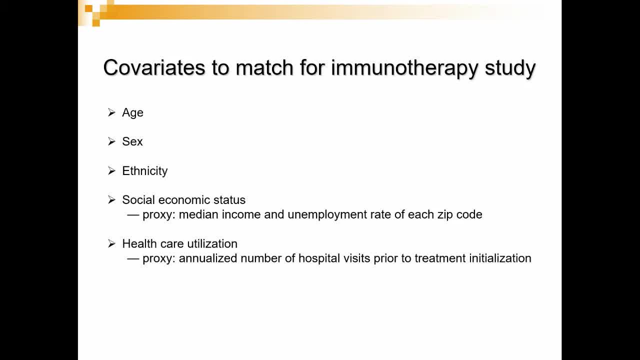 So what we use, we don't have the healthcare utilization, something called healthcare utilization, but we have a proxy- Proxy will be annualized- number of hospitals prior to treatment initialization. That gives you a number of hospitals. That gives you a way to approximate healthcare utilization. 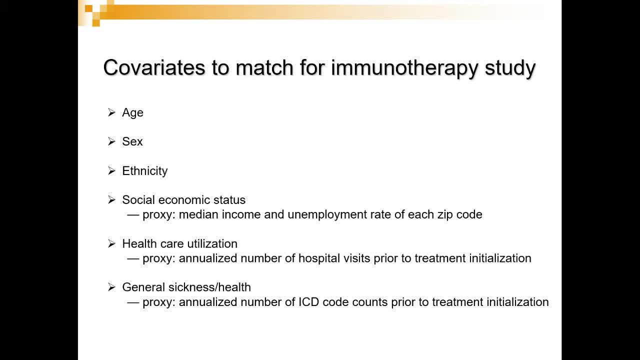 Then you also want to. the key covariate will be the general thickness of the patient. Clearly, you don't want to compare a healthy patient versus a relatively healthy patient versus a relatively poor patient And a relatively unhealthy patient. what is a proxy for that? 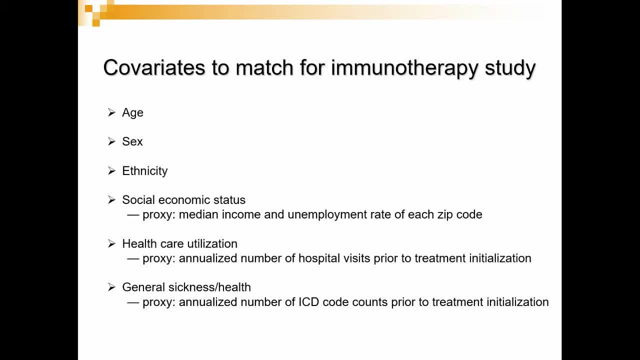 Well, we use annualized number of disease codes. disease code counts in the data set as a proxy And sick patients tend to have a lot of disease codes in the database And if you can use that to do the matching, you can do the medicine for that for this patient. 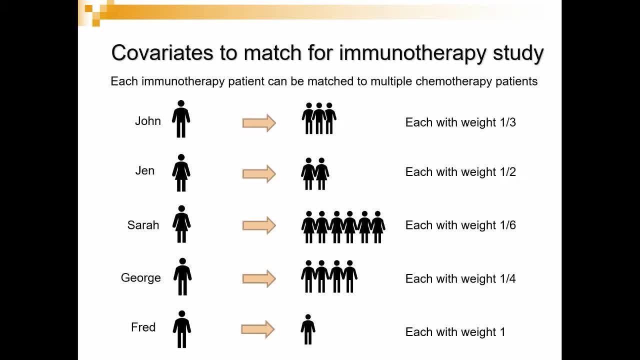 You use that to do the matching. Okay, so here's for each patient. in the immunotherapy group we can find multiple matches. We generally can find multiple matches in the control group. in the control group I mean chemotherapy group And then, for example, Sarah has six found six matches. 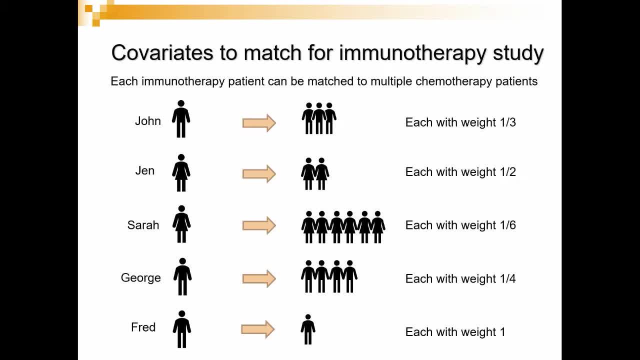 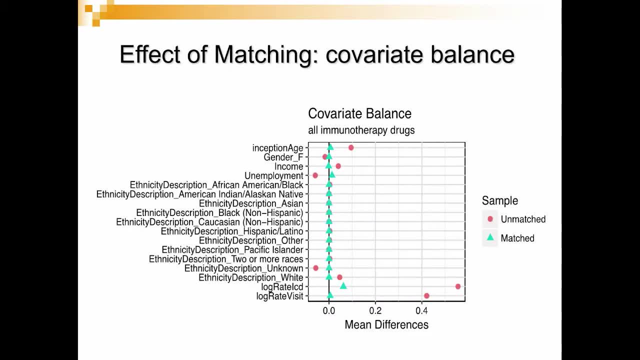 and then we assign one, six, to each of the match. So we're talking about the weighted population, matched population, but also matched control, matched treatment, control weight. And now here's the effect of matching. The red curves are what happens before matching. 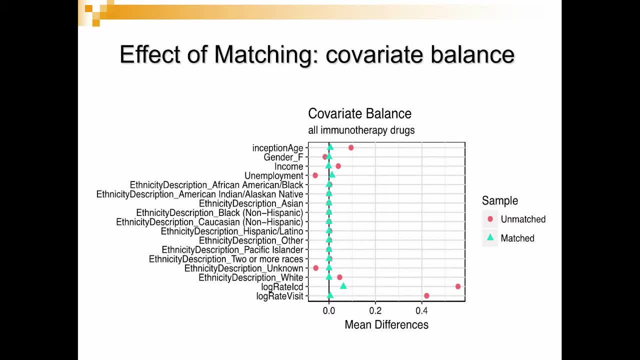 If you look at these two points, you'll realize that before matching, indeed, the treatment and control patients are very different from each other. The chemotherapy patients tend to be a lot sicker and the chemotherapy patients tend to utilize healthcare facilities a lot. 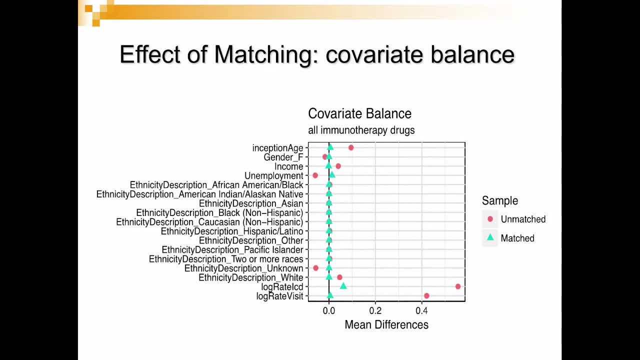 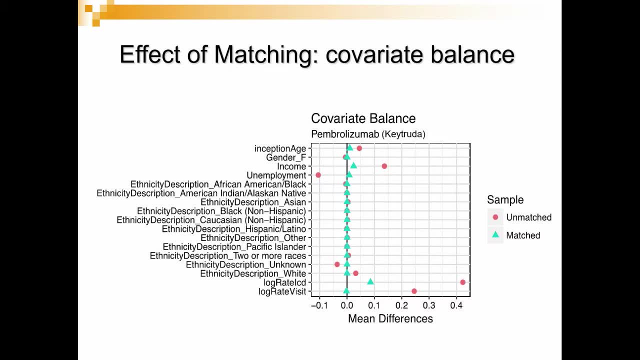 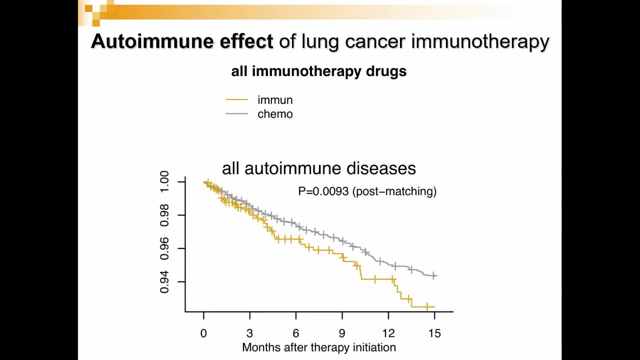 more than the immunotherapy patients. But after matching it becomes reasonable and then you can look for the individual immunotherapy drugs. Ketudar, again after matching, seems to be a lot better, And this Opdivo after matching seems a lot better. So now we can. 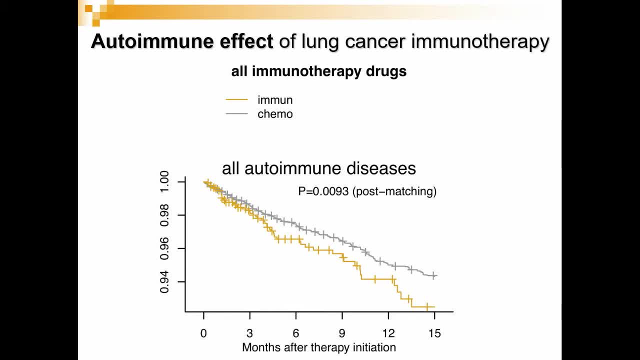 go back to study. Now we're talking about matched control pattern, matched treatment versus control with weight. Now you can calculate the Kappermeyer curve and we can also calculate the p-values. And how does this compare with the? 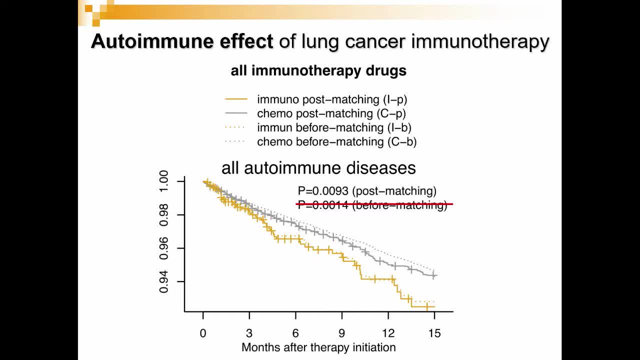 Unmatched. Well, you see that for the unmatched the p-value is 0.001, but under the matching the p-value is 0.009.. So, in other words, without doing matching, the two populations are very different from each other And you artificially generate the signal You think of 0.001, actually. 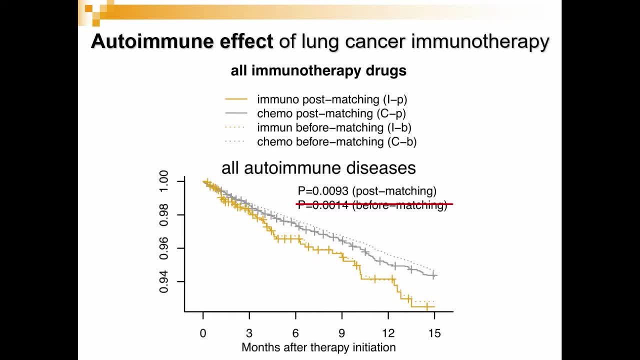 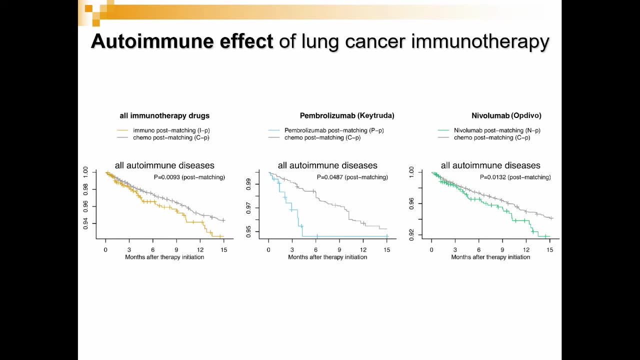 it's 0.01.. The p-value is actually 10 times as high as what you saw before, And so this is not something you want to trust. but this is more trustworthy after post-matching And we can look at autoimmune effect for individual treatment, For example, Ketudar, one drug. 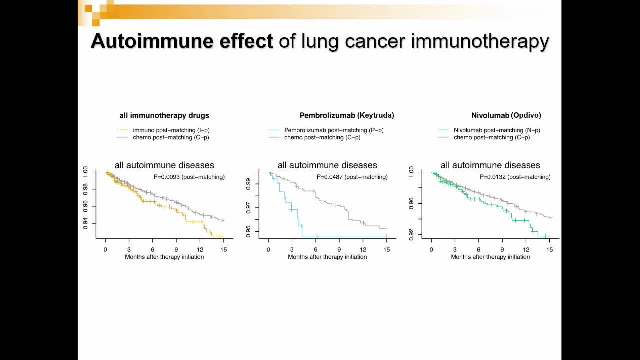 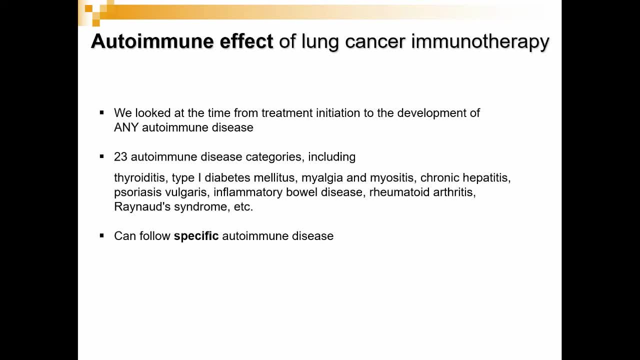 Ketudar, the other drug, Opdivo. We see, you see curves as well. you see curves. similarly, You can also calculate the p-value. Furthermore, you can talk Autoimmune disease, actually a big class of diseases. There are 23 different types, different categories of autoimmune. 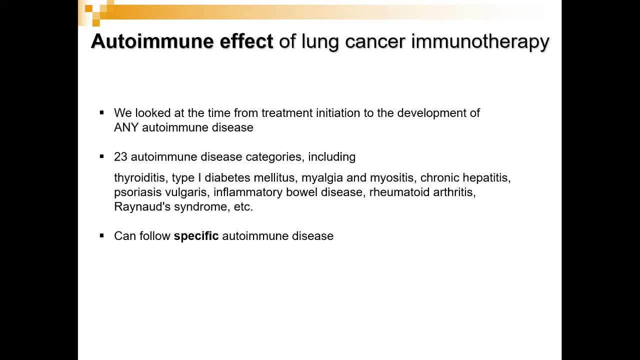 disease, from thyroiditis to type 1 diabetes, to chronic hepatitis, to inflammatory bowel disease and so on. That's actually 23 different groups categories together. So now you can look at the individual disease types and so on. Now the curves. now we have a lot of curves. 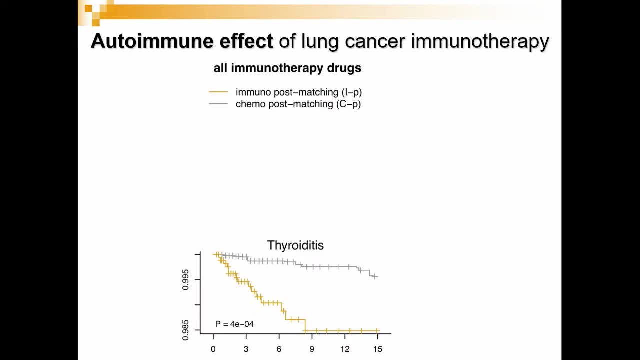 23 different individual curves to look at for different treatment. So I will, just for my time, I will just show one typical picture And out of the 23 autoimmune disease categories, 22, for the 22,, 22 out of 23,. indeed, we will observe that autoimmunotherapy has higher chance. 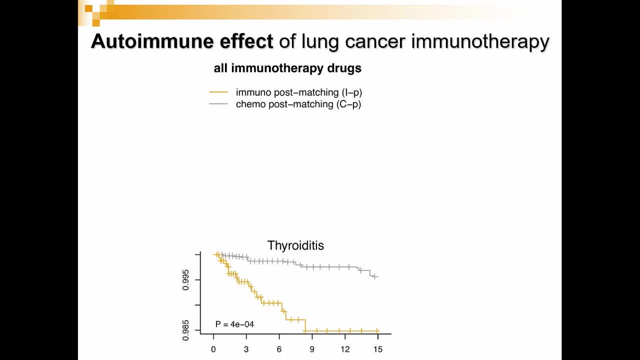 to lead to autoimmune disease. Out of 23,, 22 of them have the effect like this. Thyroiditis is the most pronounced In this case. this is a. this is a Kaplan-Meier curve for immunotherapy. This is a. 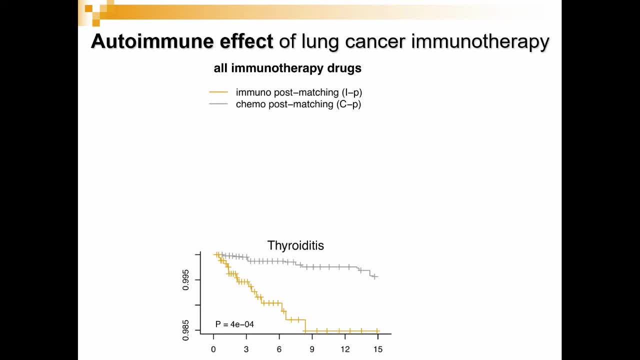 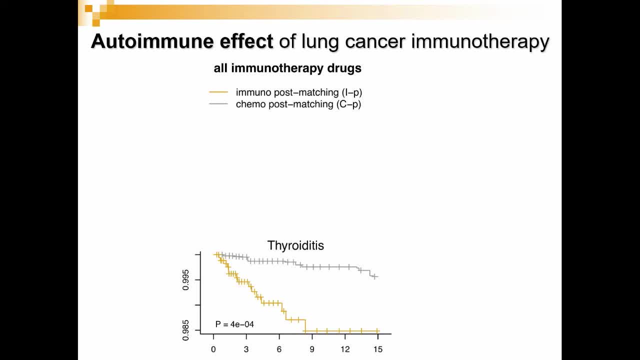 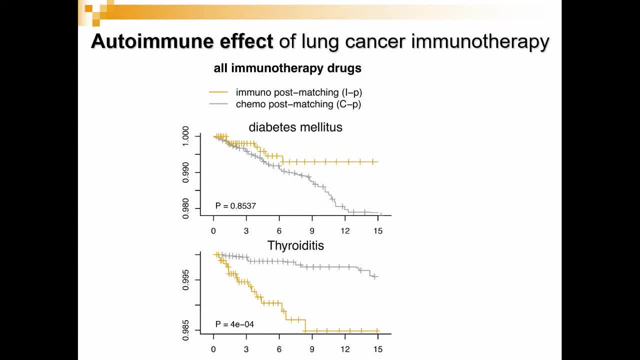 that's the only case that the, the, the relation between the two curves flipped over, So we have less type 1 diabetes incidence from immunotherapy patient versus the chemotherapy patient. Actually, this can be well explained by a well-documented side effect: The pancreatitis. 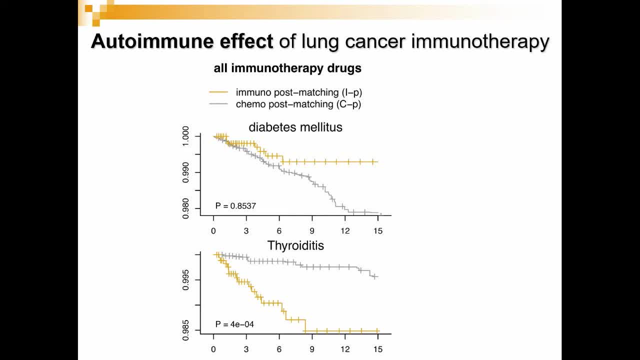 toxicity can be explained by the pancreatitis toxicity. Actually, this can be well explained by well-documented side effects. The pancreatitis toxicity is the side effect of the pancreatitis toxicity for chemotherapy. that's well documented. and then chemotherapy disrupts the blood, the blood sugar homo status, so this can well be attributed to. 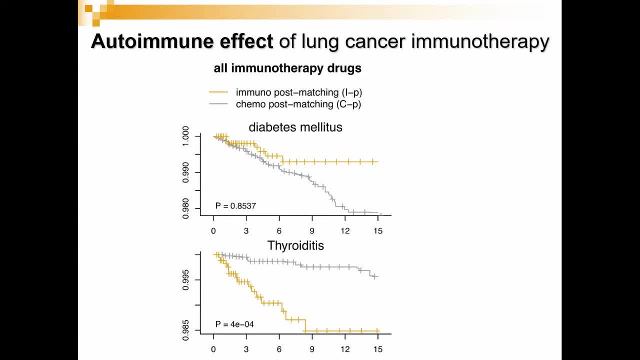 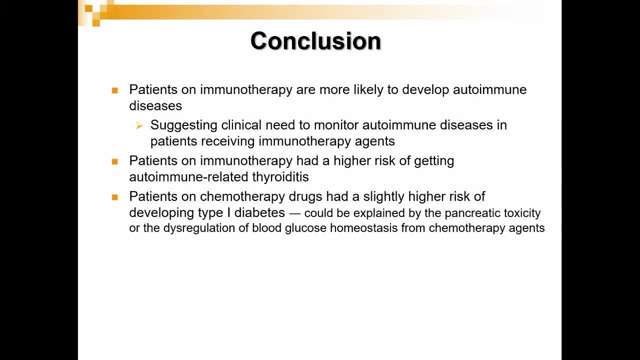 this specifically: doctor already noted effect of chemotherapy. okay, now my time is up, so let's sum up. sum up so what we find. based on this large data set, patient immunotherapy are more likely to develop autoimmune disease. so this essentially suggests that when doctor do immunotherapy for cancer patient 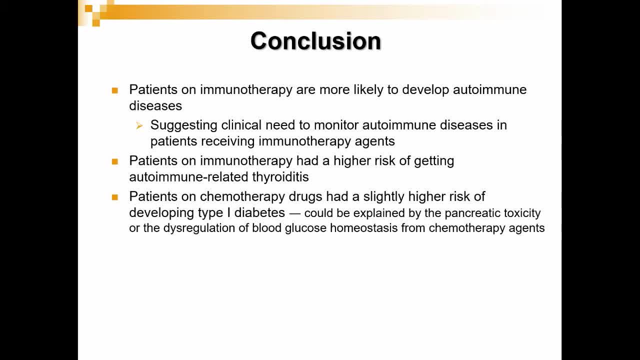 doctor should watch out for immunotherapy consequences should pay attention. and secondly, immunotherapy generally have a high chance. immunotherapy in terms of specific disease. immunotherapy treatment had a higher risk of getting autoimmune related thyroiditis. on the other hand, a patient on chemotherapy had the slightly higher chance of developing type 1. 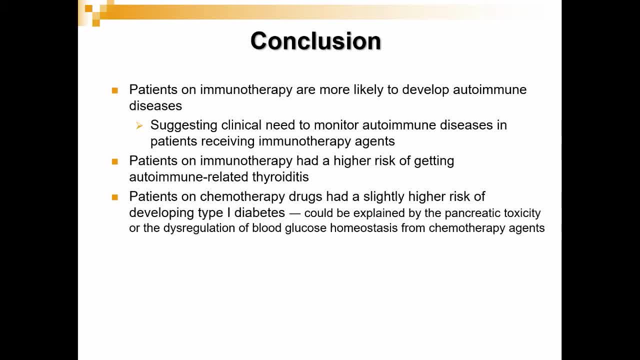 diabetes. that's what we found. what do we observe from data set? to draw conclusion, I, in my, this is my adventure in, this is my, our adventure in the big medical data- and we do think that big data presents a great opportunities, especially to study real disease, real treatment or emerging treatment, in this case, cancer. 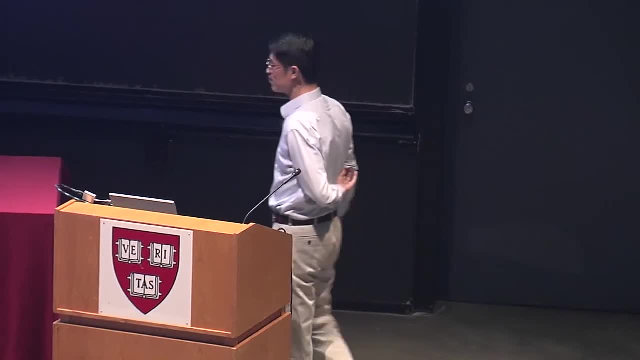 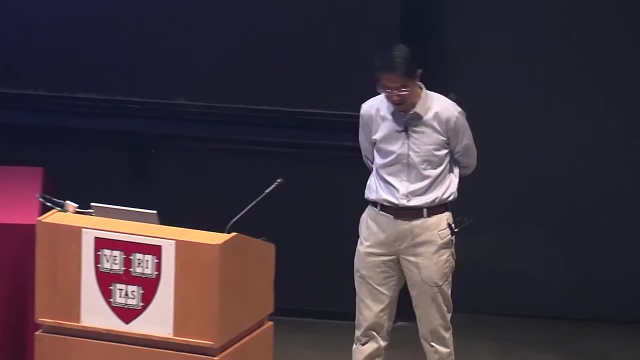 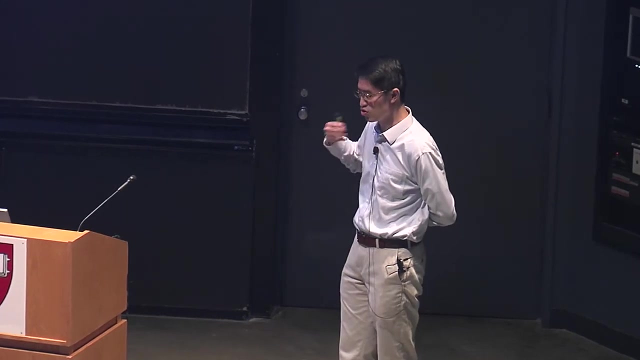 immunotherapy and I also want to say that size does matters: 44 million make a big difference from like 1,000 patients and so on. but in my opinion, the careful and analysis, careful status, analysis and careful thinking really makes, makes critical difference for you to draw reliable, trustworthy conclusions. thank, 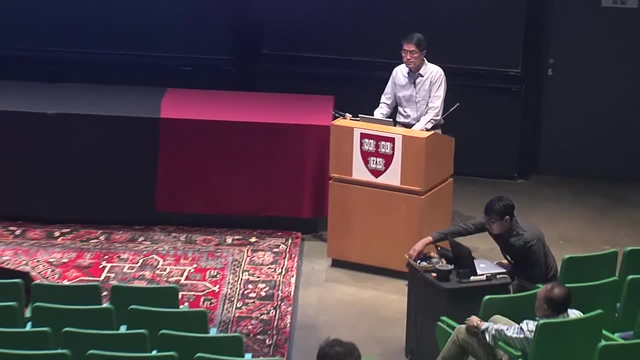 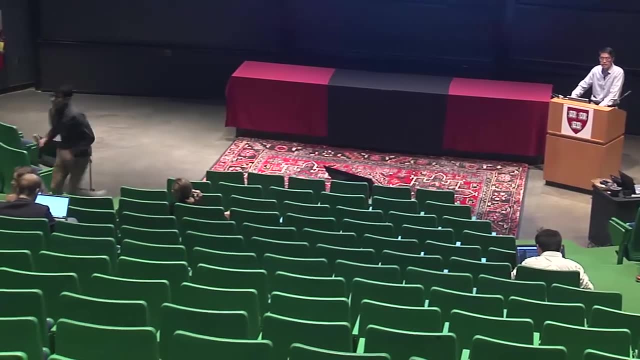 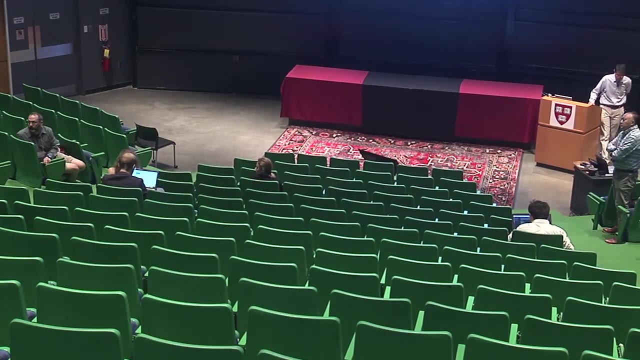 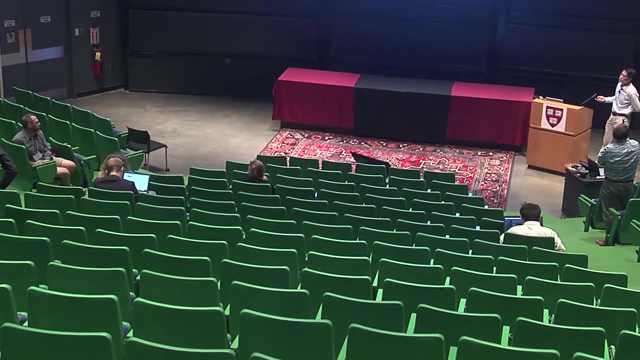 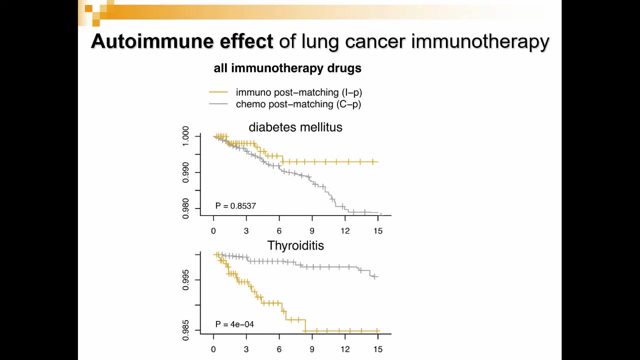 you very much. thank you, I know how are you some, so I have a couple of questions. yes, thank you very much. if you go back a couple of slides, well, even there- the lower one, this- the effect size is very small in most of the y-axis on your plots, do I mean? I know that 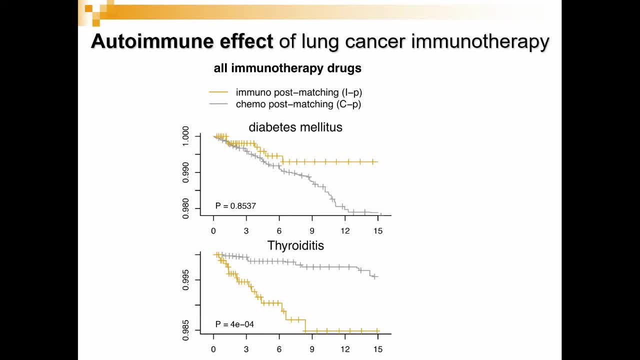 you've done this physical analysis and it shows that the both populations are distinct, but is not a meaningful if you, as a patient, were treated with one of threatened because you go from 0.995 to 0.001,. you know what I'm saying. 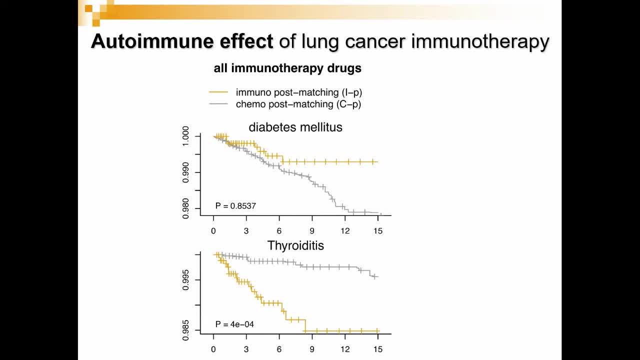 Yeah, this is actually not a long for us If you read all the medical journals- and people typically don't present this type of picture. it's something called odds ratio, Right? That's basically the ratio between 0.001 versus 0.00001.. So basically, you see like one tenfold. 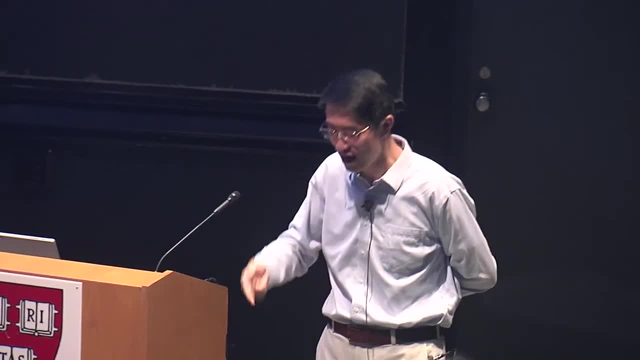 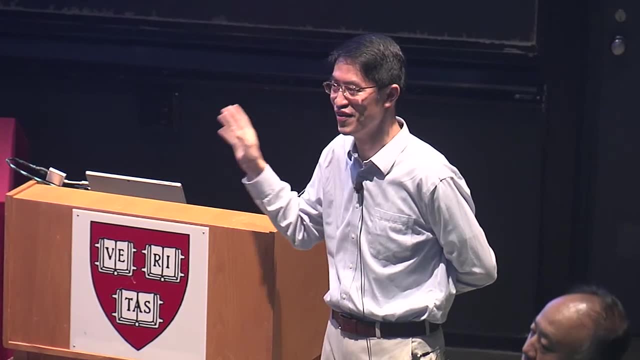 odds ratio. If you see an odds ratio above one, significantly above one, chances are that if you talk about some disease, chances are you can make it to New England Journal of Medicine or JAMA. That's not our story alone. That happens pretty prevalent in all the medical journals and so on. 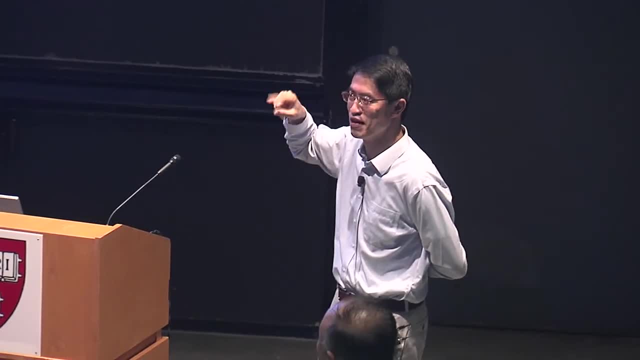 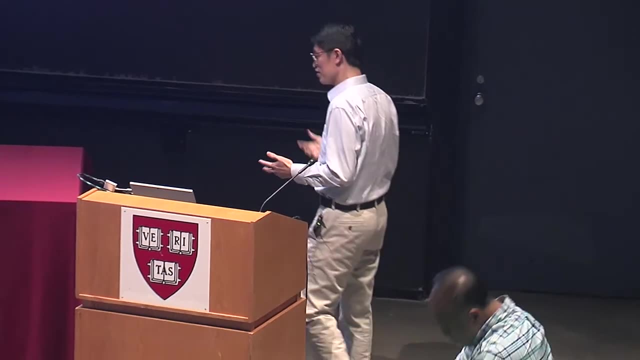 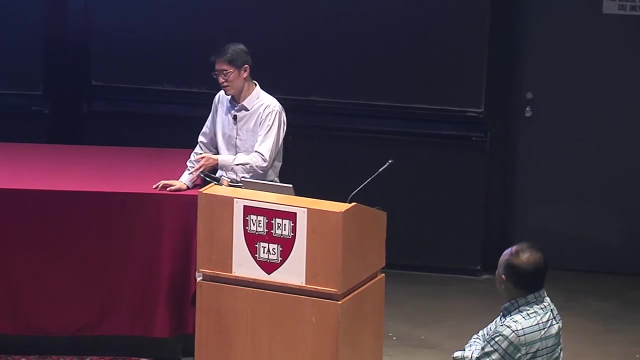 So you're looking for even above one, significantly above one odds ratio. So in this case I would say, depending on what your expectation about this. Of course you're talking about the life-threatening condition, Even if you get for a patient, if you are talking about whether you want to live or die. in three months versus you're got an immune response, autoimmune disease in three months probably. I would depend on each individual patient choice. The doctor would suggest yes, even if you want to develop, you might get a chance to develop autoimmune disease. maybe you want to still go for. immunotherapy because that might save your life. But later on you should inform the patient that you have a higher chance. They have a higher chance of developing autoimmune disease versus classical chemotherapy. So you shouldn't be surprised if later on you develop thyroiditis and so on. So that's actually the story about all the medical studies. 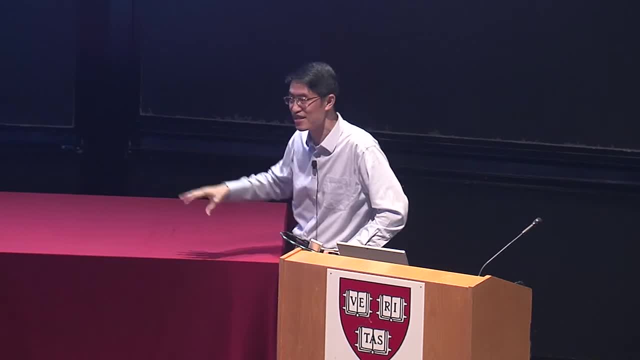 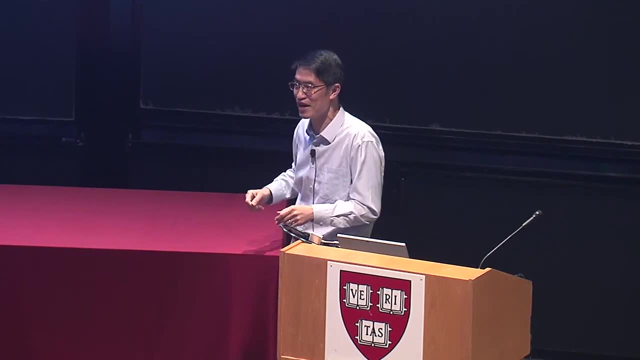 As a matter of fact, if you study the relationship between smoking and lung cancer, you see stuff like this also. And you smoke for five years. the chance of developing lung cancer is minute. But we all know we should avoid smoking. We all know smoking causes lung cancer, So that's. 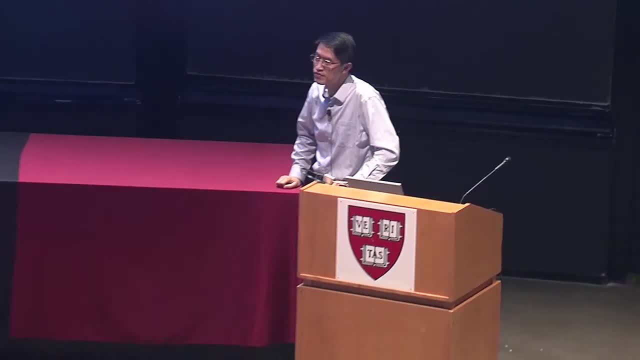 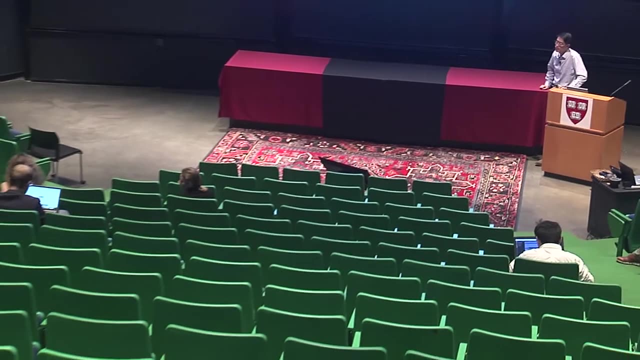 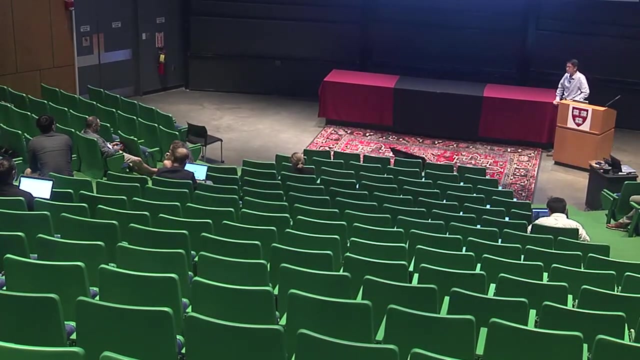 a long story here, Right, And so the second question and then the third question which I think is really important is: in the medical community, the reputation of electronic health records is that they are very good at tracking billing, meaning they're very good for hospital management. But in principle people record ICD codes. 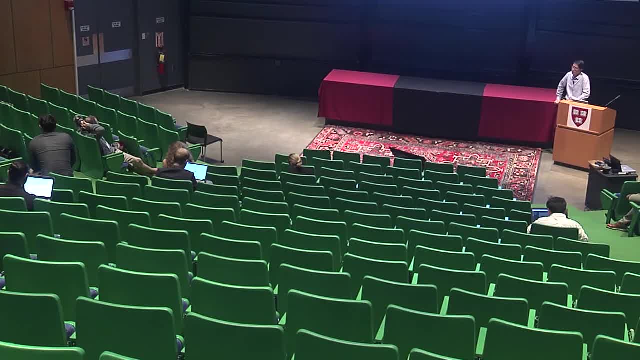 which are describing whether a patient has a specific disease in ways to protect the hospital from spending more or less money as opposed to accurately what a person is, you know, describing the person's health. So I wonder how you guys are planning on, because reviewers and even the general public, who 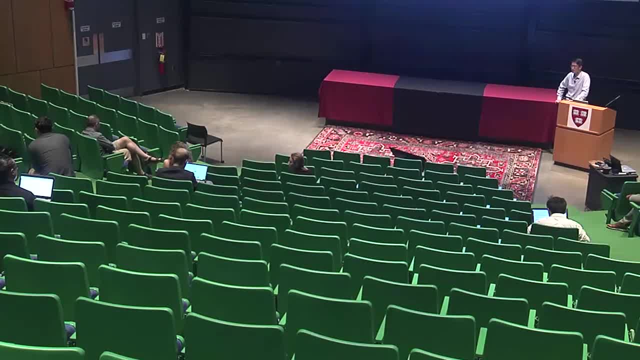 knows about this. how do you defend your study and say, well, you know this matching, it's a great methodological piece, but perhaps on data, that has a bad reputation. that's what I'm like. Well, that's actually a good question. 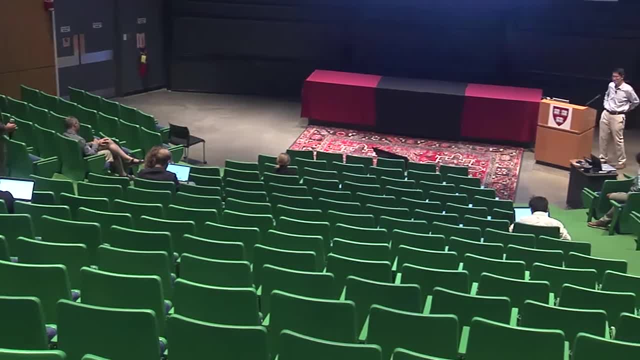 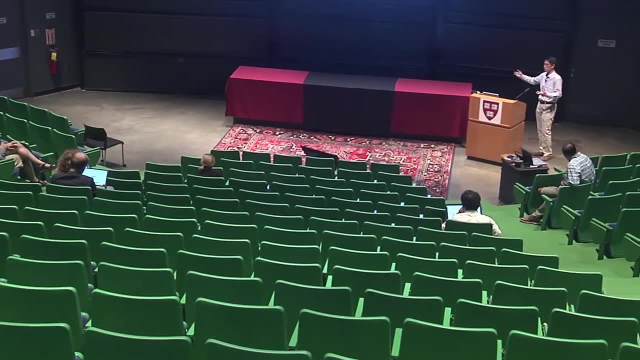 The electronic health record or medical insurance data like this. it was not designed for research, for us to study disease. the Q or association. The original idea is to for efficiency of processing internal processing hospital. for the doctor enter your patient ID and so on. Then you 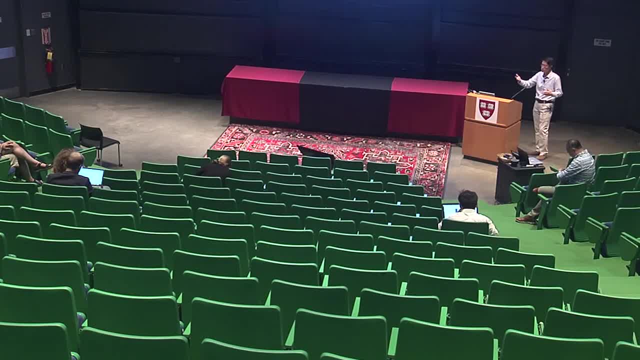 get all your past record treatment in the same hospital. That's our initial design, But a side consequence, or a good part, is that it also opened up if you want. of course you have to anonymize, protect the patient privacy and so on, but it opens. 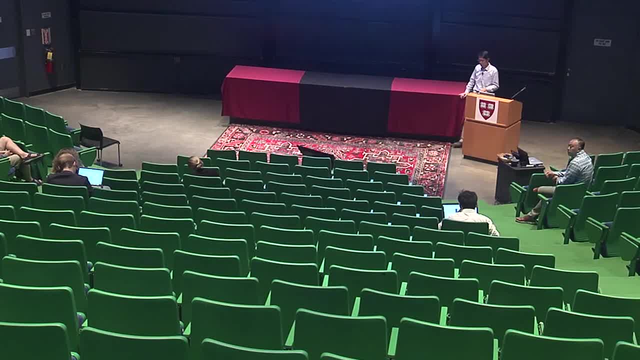 your door to access a large amount of information, And that amount of information can well lead to novel medical treatment, novel discoveries and that can prevent disease and so on. So I think that's actually a good part of electronic health record and medical record. 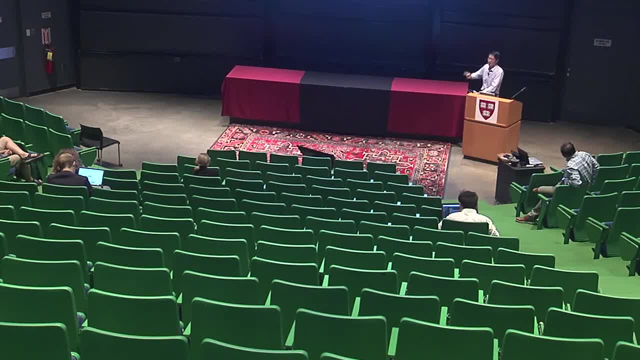 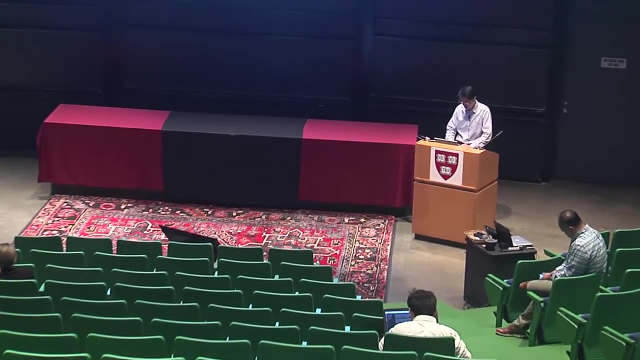 And specific, as you said, and that was in the details, right, And so in this particular case, we have a very simple question: What is a lung cancer patient? How do you define lung cancer patient in this case? Because that's actually related to what you say, what the question is. 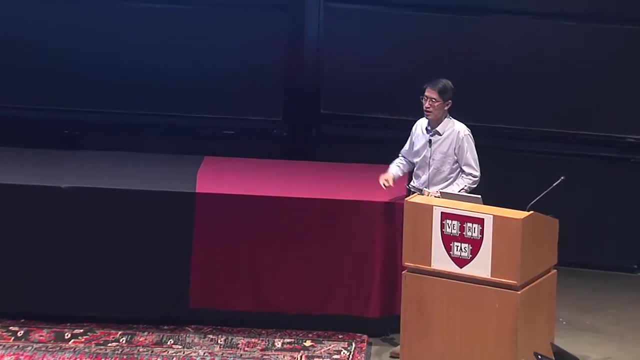 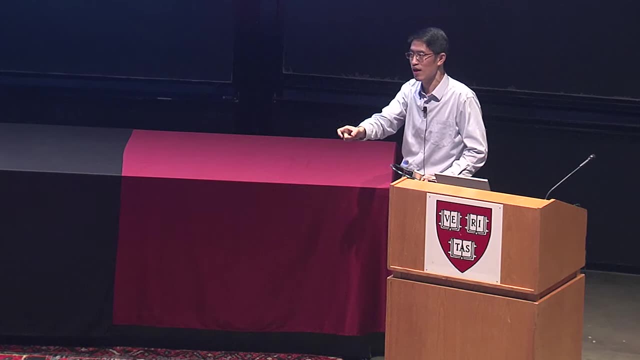 If you look at the insurance data set, this only talk about disease code. They only talk about disease procedure code and medication code. There's no column to say this guy is a lung cancer patient and that guy is not a lung cancer patient. Actually, there's also no dimensioning of whether 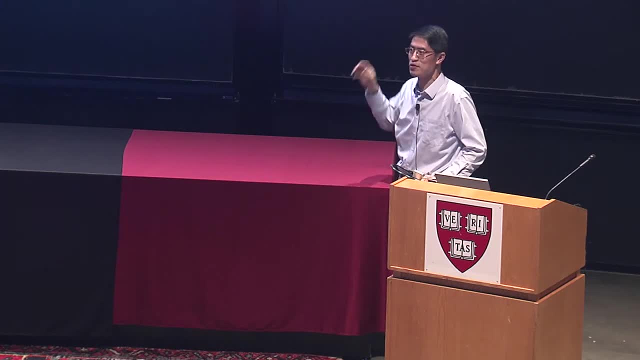 this guy is an autoimmune disease patient. that guy is autoimmune, So you have to find out. so how do you find this? How do you identify who is lung cancer patient That has that? actually something has to go behind it, And it's not just this guy. this guy did a. 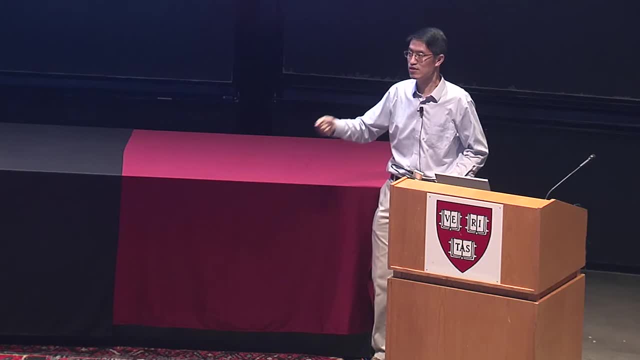 lung autopsy then therefore, this guy is lung cancer patient. The answer is no. This guy might be a healthy guy, just the doctor suspect something. In the end the results shows different, Then this shouldn't be treated as lung cancer patient. So you have to be careful about even 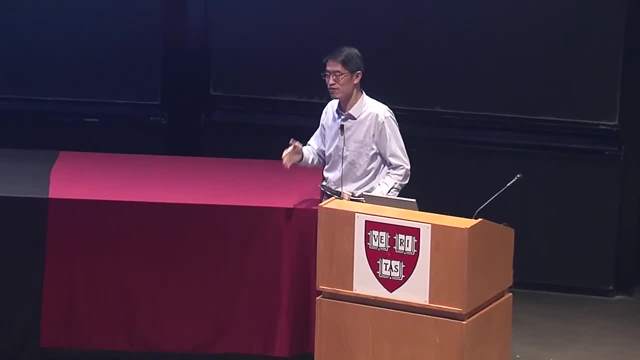 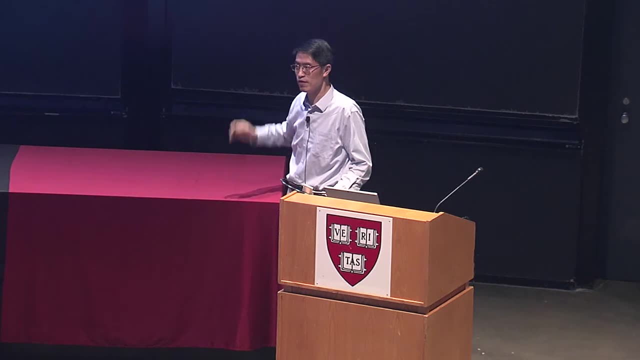 the definition of lung cancer patient, your definition of the chemotherapy patient, your definition of immunotherapy patient as the same thing. So when you deal with this type of data, you have to be very careful. For example, this is our logic of identification of lung cancer patient. It's not just mentioning 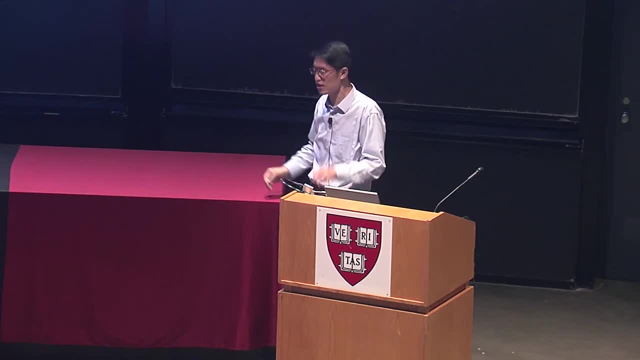 ones. Just not only talk about diagnosis criterion. Actually there are diagnosis criterion, procedure criterion and pharmacy criterion. So our definition is that at least you have to observe three independent claims meeting one of those criterions or two mentioning of the criterion. 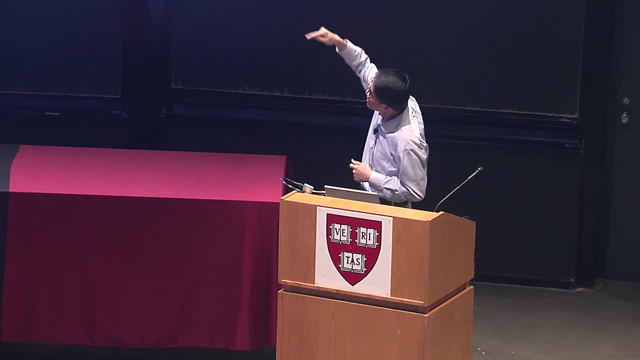 two independent claims recalls in at least two separate groups that give us confidence. what indeed? talking about the lung cancer patient, Another case will be have to be very careful. What starting the caudal effect? So you want to rule out all the patients that already have? 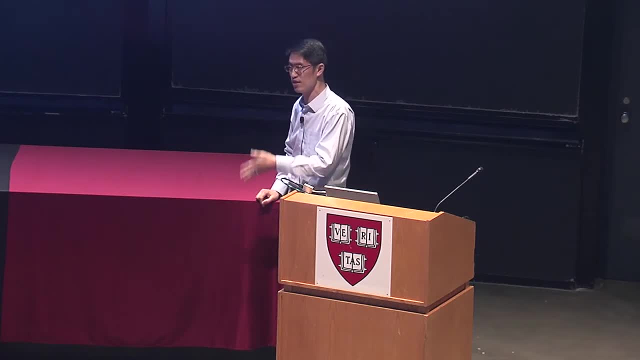 autoimmune disease, Then you cannot. obviously you cannot see this is caused by cancer treatment. So when you define the patient cohort, you have to rule out all the patients that already have autoimmune disease. So that has been ruled. Another thing has to be ruled is that what if this patient is new to this insurance database And then from the first week the patient start to receiving cancer treatment, Then for this patient you also want to be careful because maybe this pre prior to joining this new insurance plan, the patient already have started cancer treatment. So you want to have a quiet period, that indeed, for the first two or three months, nothing going on. Then you're confident that this is actually new lung cancer patient rather than a lung cancer patient already struggling with lung cancer for three years in the back. 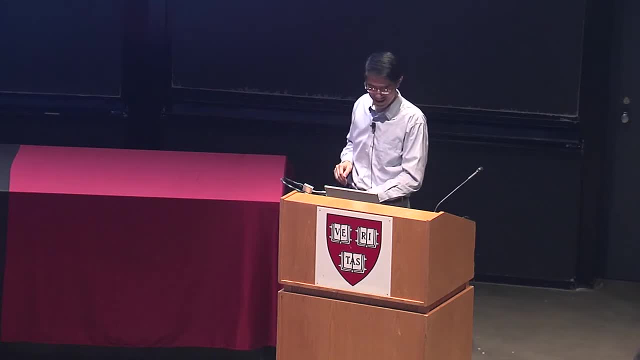 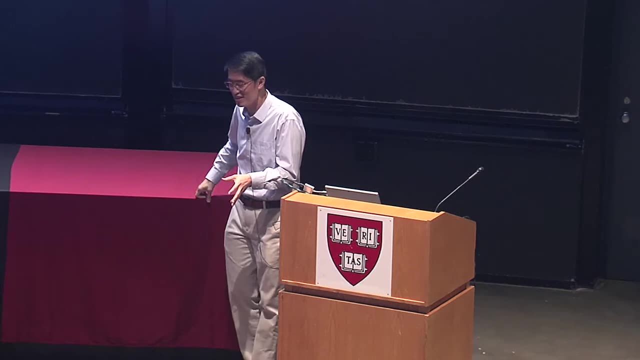 So that's a lot of nitty gritty details for this type of things And, okay, this exposure and so on. So, indeed, the data messy, but pre-processing understanding what I'm looking for- that actually takes months for you to investigate the data set. So data is dirty, Data is not clean. 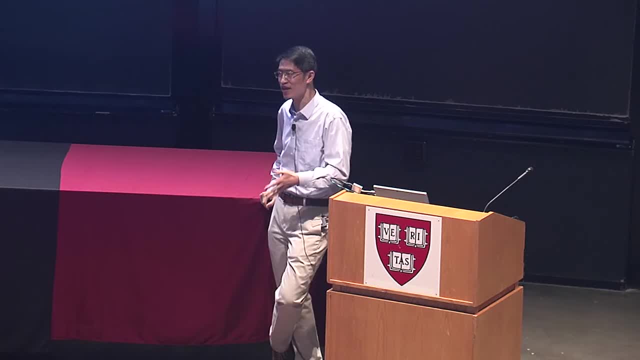 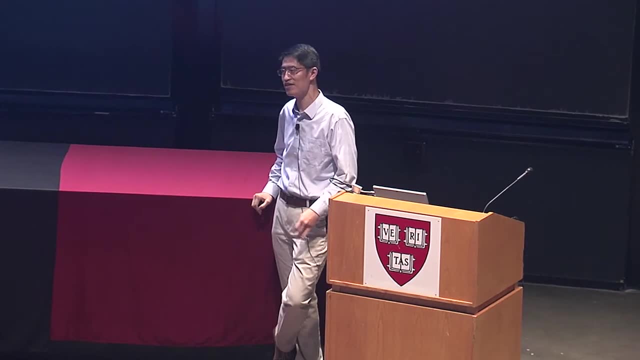 And, as a matter of fact, you spend 40 or 50% of effort cleaning the data. try to understand what is the data. how do you extract all the information? Then you can carry out the status analysis. So the answer is that this data is not well prepared for. 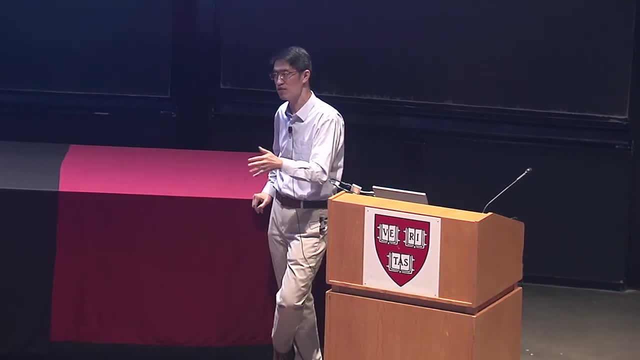 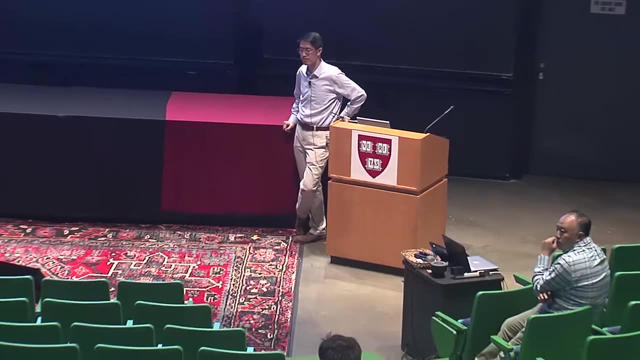 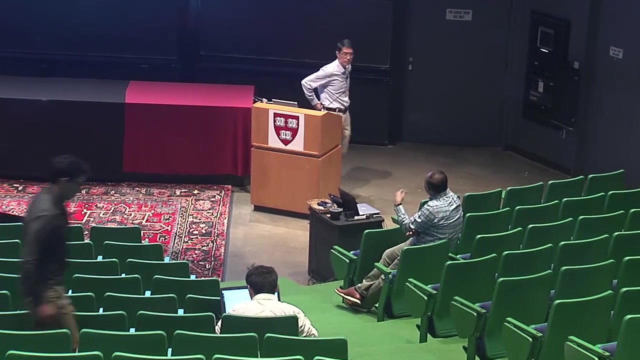 research. If you want to do research there, you have to be careful, You have to do a lot of pre-processing and pre-study and so on. Yes, Can you quickly factor how, the? what's the effect, whether it's indeed better than chemotherapy? 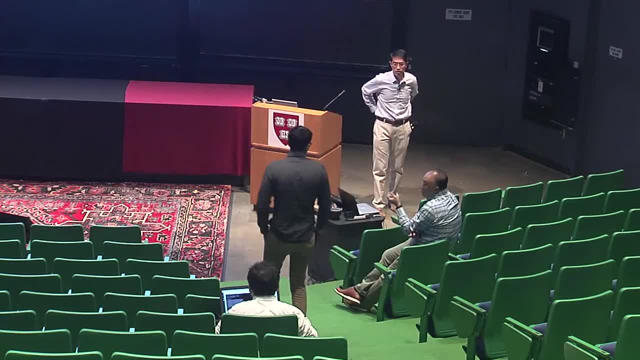 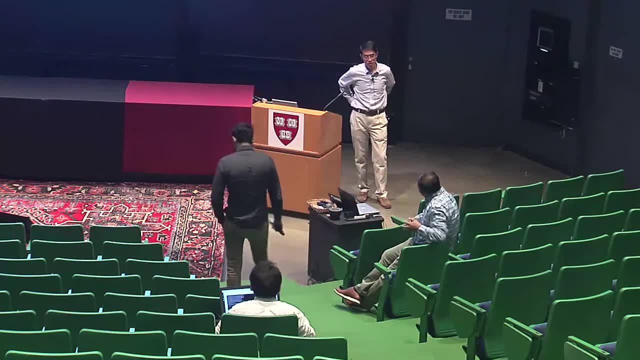 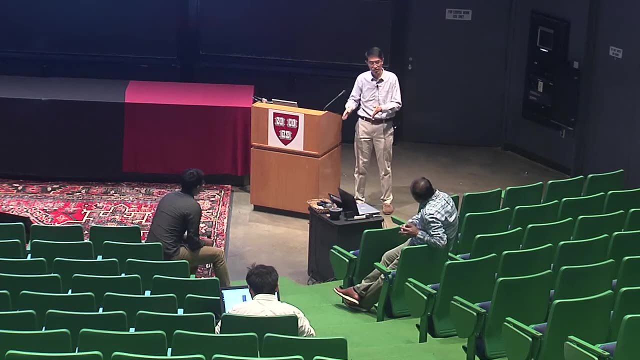 to the response to relapse. Oh yes, that's indeed, That's actually already. that's what FDA. when FDA approves the drug, you have to do double-clinic. In terms, there's different measurement: First, prolong the patient's life or reduce the tumor size. 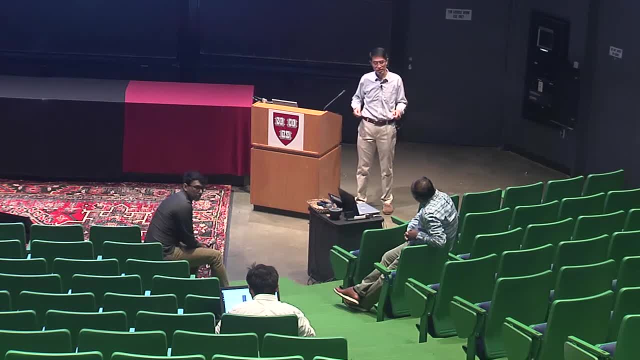 In. both are reported and both actually for Keytruda for example. that's report. there are two clinical trials, two studies reported in the New England Journal of Medicine And also journals, those articles reporting Lancet and so on- that basically talk about the clinical trials before the drug get. 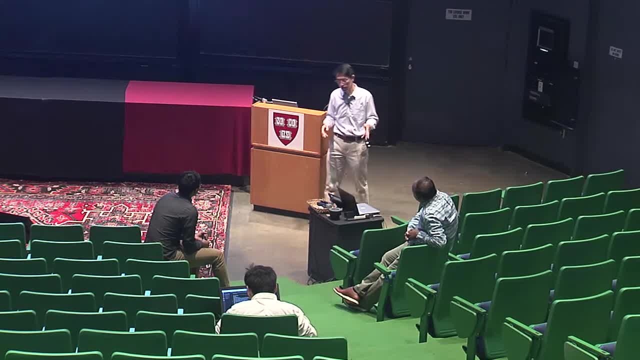 approved by FDA. They do run a clinical trial, But the clinical trial typically you involve less than 100 patients, But the clinical trial typically you involve less than 100 patients. Unfortunately that maybe wouldn't go rid of the ample time any patients were. given at risk of relapse. In your range, which is directly employment, Are the risk to relapse at least, on average, 10 times less. I believe. that's, I guess大概 20%, 35 times less in the full length of the service. 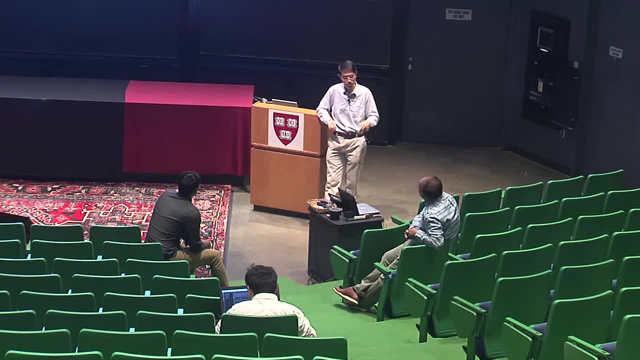 Three times over In three months, more, maybe less, Same for the contracting three months or six months or something like that. But that's also a problem with we also have a strong censoring going on. So all the drugs pretty much. 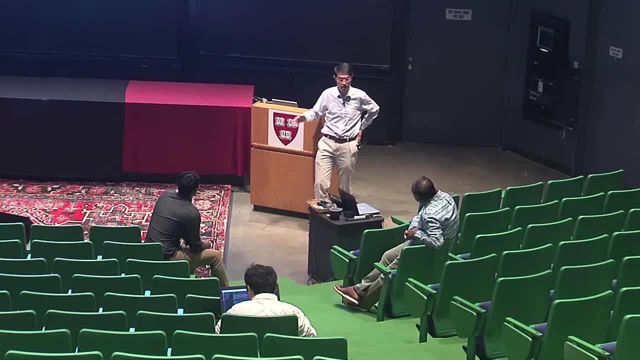 you see, the vast majority of the data we have is from 2016 onward, So now we only have two years afterward. before that, We have a lot of censoring going on. So our estimate is based on the censoring and so on. 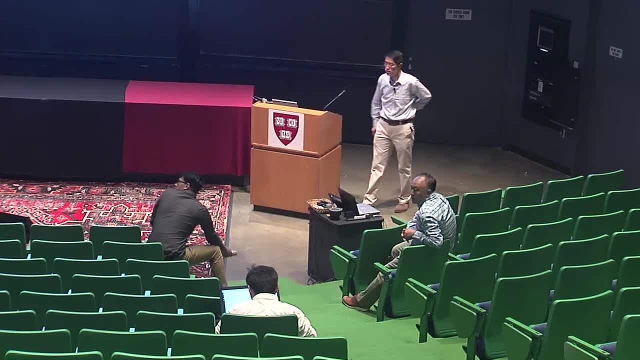 Okay, so that's the end of this morning session. thank you. 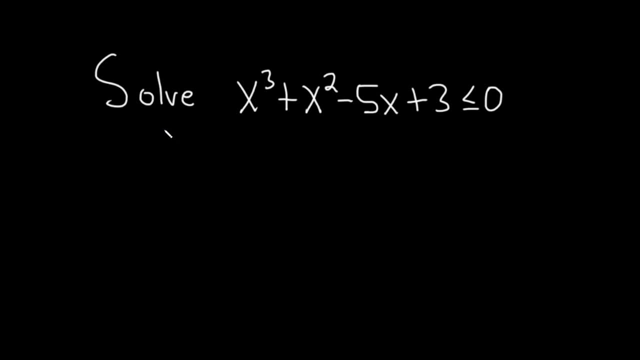 Hello, in this problem we have to solve this inequality. So we have x cubed plus x squared, minus 5x plus 3, and that's less than or equal to 0 solution. So let's go ahead and see what we can do here. We have four terms and we somehow have to factor.